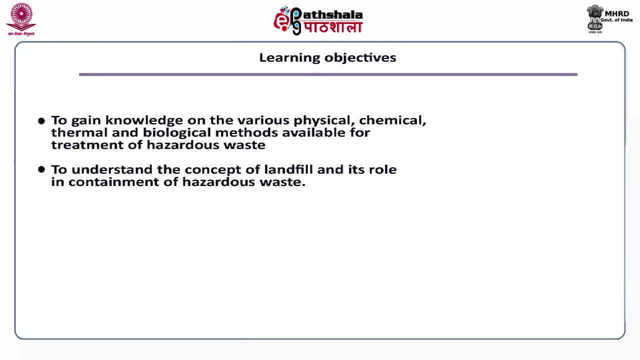 Second, to understand the concept of landfill and its role in containment of hazardous waste. Third, to familiarize the alternate disposal options available for hazardous waste. Now treatment and disposal. So for treatment and disposal, hazardous waste reduction and minimization is of foremost importance. 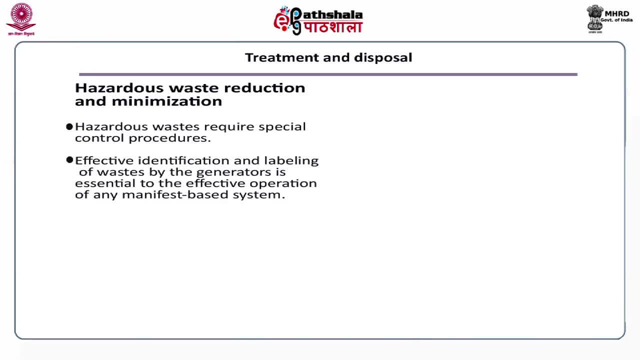 Hazardous waste requires special control procedures. Effective identification and labeling of waste by the generators is essential to the effective operation of any manifest-based system. Management of hazardous waste implies consideration of alternate methods and schemes, both institutional and technical, to hazardous waste reduction. 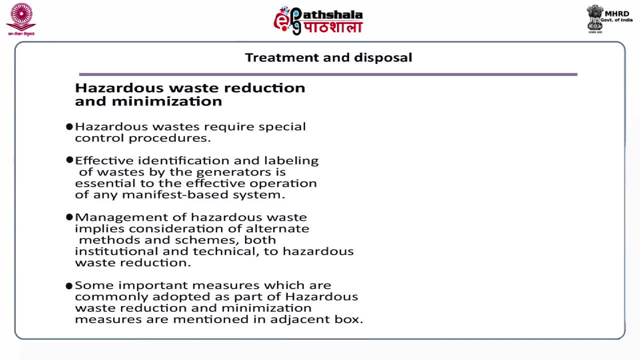 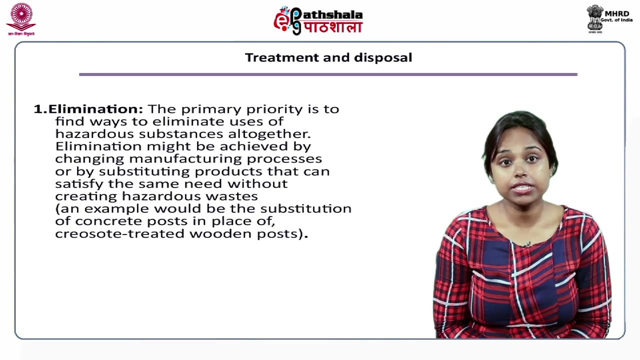 Some important measures which are commonly adopted as part of hazardous waste reduction and minimization measures are mentioned in adjacent books, Which includes elimination, reduction, recycling, Treatment to reduce their volume and toxicity. First, elimination: The primary priority is to find ways to eliminate use of hazardous waste. 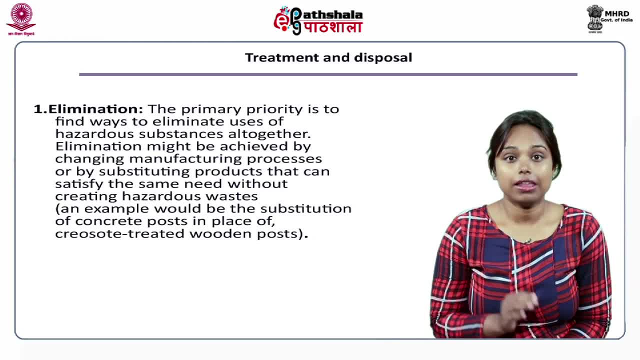 eliminate uses of hazardous substances altogether. Elimination might be achieved by changing manufacturing processes or by substituting products that can satisfy the same need without creating hazardous waste. For example, substitution of concrete post in place of creosote treated wooden post. Now reduction. 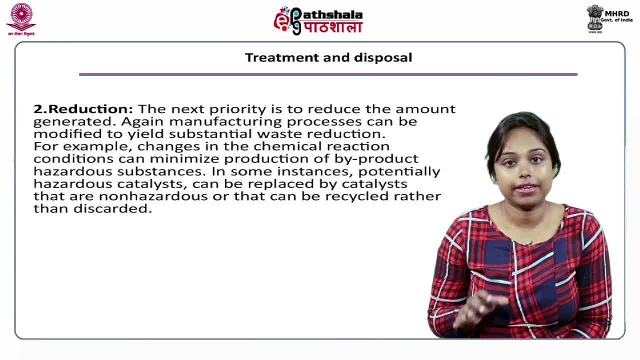 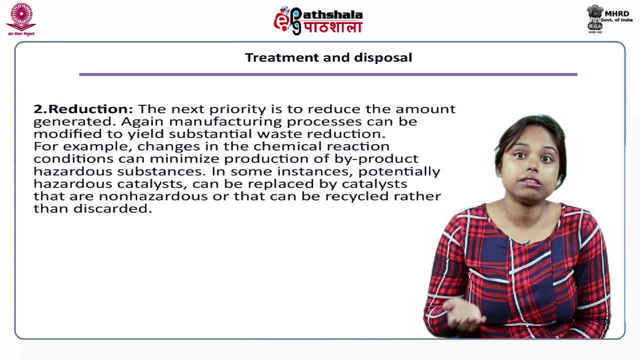 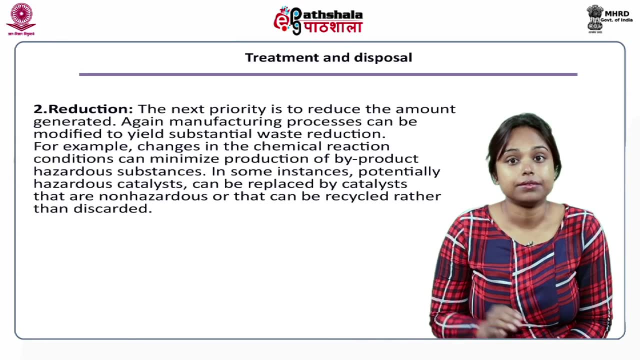 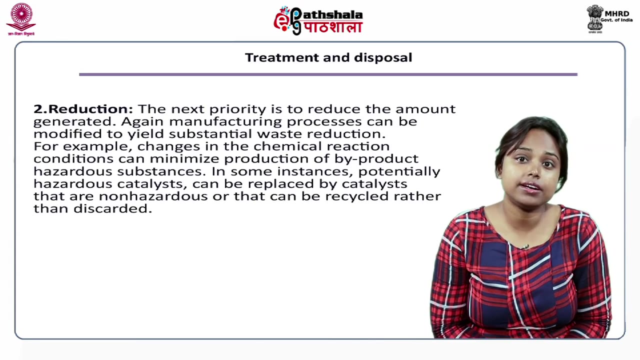 The next priority is to reduce the amount generated. In addition, manufacturing processes can be modified to yield substantial waste reduction. For example, change in the chemical reaction conditions can minimize production of byproduct hazardous substances. In some instances, potential hazardous catalyst can be replaced by catalyst that are non-hazardous. 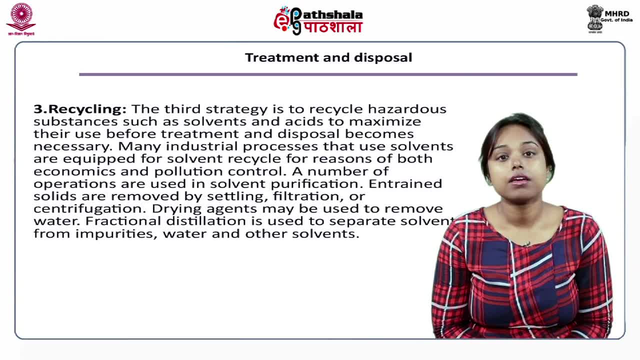 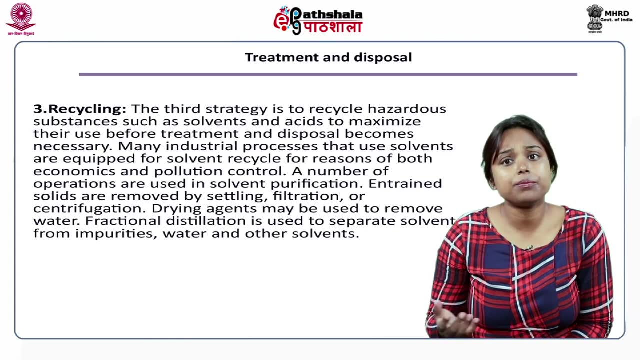 or that can be recycled rather than discarded Now recycling. The third strategy is to recycle hazardous substances, For example, the use of hazardous substances such as solvents and acids to maximize their use before treatment and disposal becomes necessary. Many industrial processes that use solvents are equipped for solvent recycle for reasons. 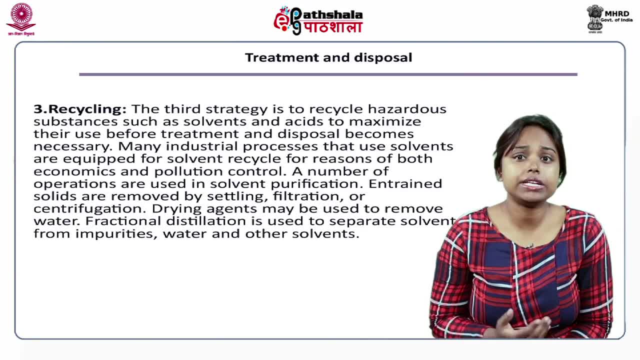 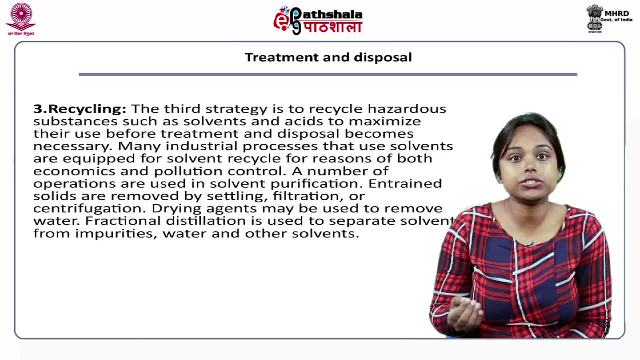 of both economic and pollution control. A number of operations are used in solvent purification. Entrained solids are removed by settling, filtration or centrifugation. Drying agents may be used to remove water. The next priority is to reduce the amount generated by hazardous substances. 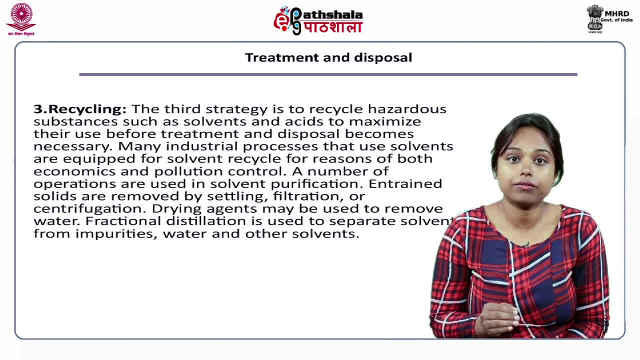 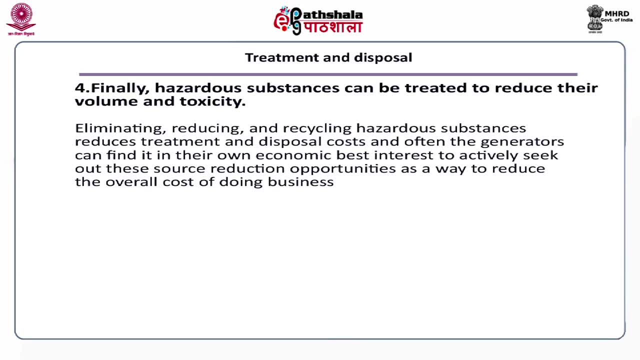 Fractional distillation is used to separate solvent from impurities, water and other solvents. Finally, hazardous substances can be treated to reduce their volume and toxicity. Eliminating, reducing and recycling hazardous substances reduces treatment and disposal cost, and often the generator can find it in their own economic best interest to actively seek. 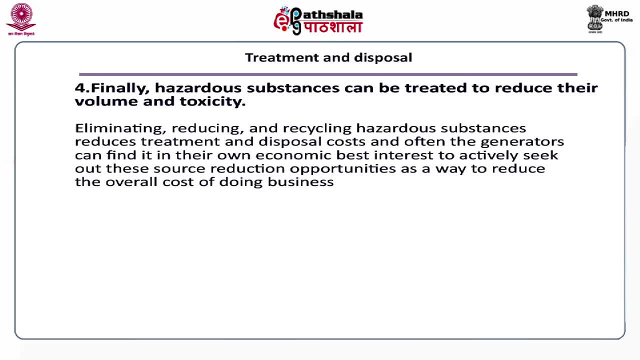 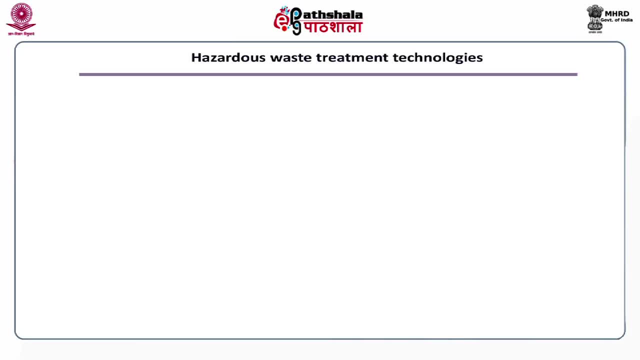 out these source reduction opportunities as a way to reduce the amount generated by hazardous substances, Now Hazardous Waste Treatment Technologies. The selection of the treatment process for waste tree depends on, among other factors, the nature of the waste desired. characteristics of the output stream. 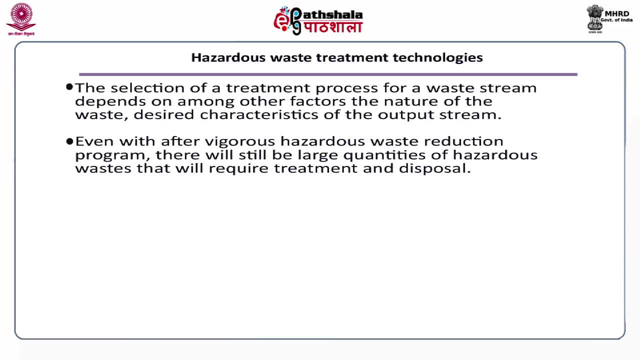 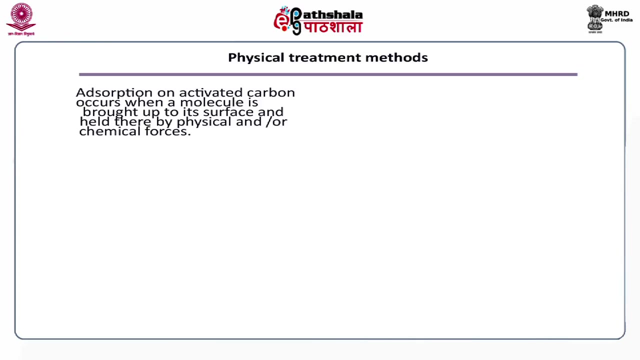 Even with after vigorous hazardous waste reduction program, there will still be large quantities of hazardous waste that will require treatment and disposal. The treatment technologies have been characterized by the use of hazardous substances in the yet-to-be- темперatrable materials, such as actual muitalakotene and 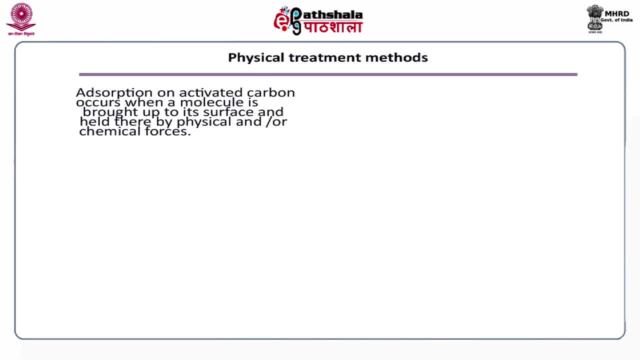 世 pelvis. If the contact surface is uninhabitable, it is przeklenged, and бли McG authored byptillaud To preserve revenge on causes and treatments. in the case of worriest natural precipitations, the treatment process must be made sustainable. Factored positions have been characterized as physical®, chemical, biologicalthermal. First physical treatment method. Under this comes the first absorption. Absorption on activated carbon occurs when a molecule is brought up to its surface and held by physical or chemical forces. This process is reversible, thus allowing activated carbon to be regenerated and tantalized. This is the first collaboration of aNoturel, not a carbon to be 돌아ed. This is how vår main energy of attention occurs. after annihilating organic acids, Consequently tablespoon of the chlor, wiggle is nature. Under these processes needed堅60 steric. Gracias to all. Thank you for watching. 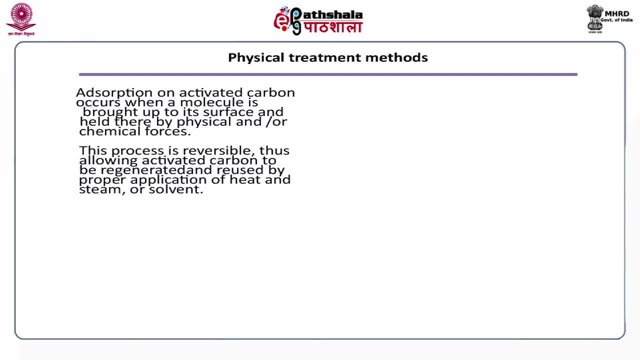 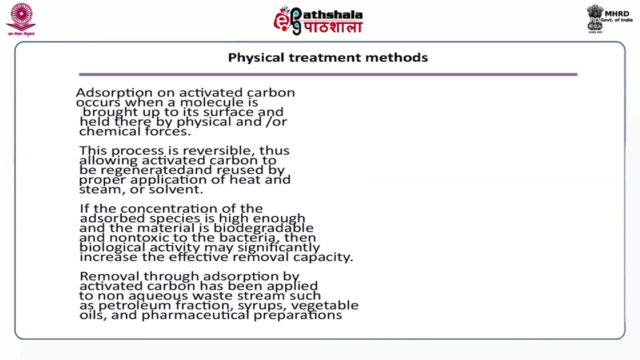 reused by proper application of heat and steam or solvent. if the concentration of the adsorbed species is high enough and the material is biodegradable and non-toxic to the bacteria, then biological activity may significantly increase the effective removal capacity. Removal through adsorption by activated carbon has been applied to non-aqueous waste streams. 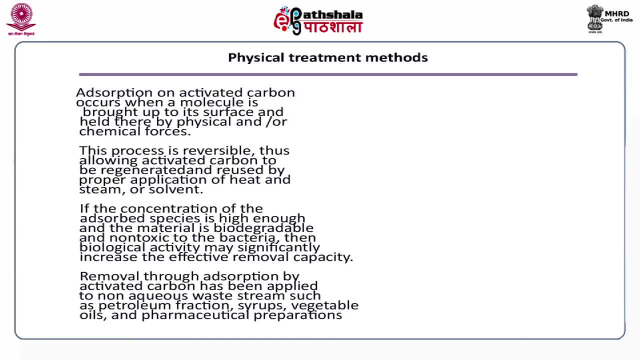 such as petroleum fraction syrups, vegetable oils and pharmaceutical preparations. The factors that relate to adsorption capacity are: greater surface area produces greater adsorption capacity. For example, activated carbon has large surface area. Absorptivity increases as the solubility of the solute decreases. 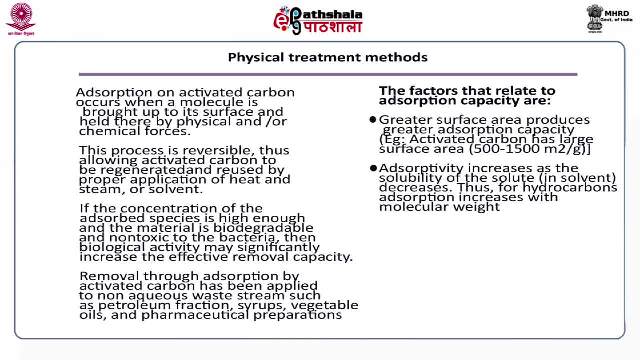 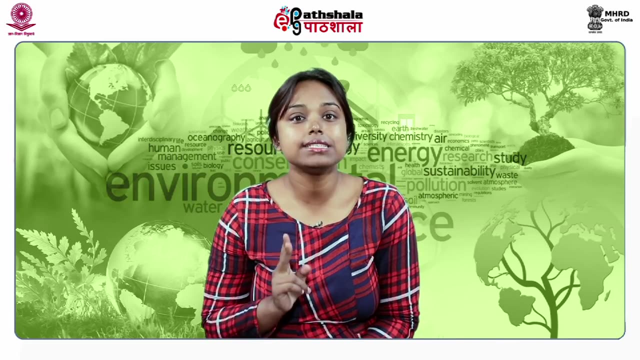 Thus, for hydrocarbons, adsorption increases with molecular weight. For solutes with ionizable group, maximum adsorption will be achieved at pH corresponding to minimum ionization. Adsorption capacity decreases with increasing temperature. Now resin adsorption. Waste treatment by resin involves two basic steps. 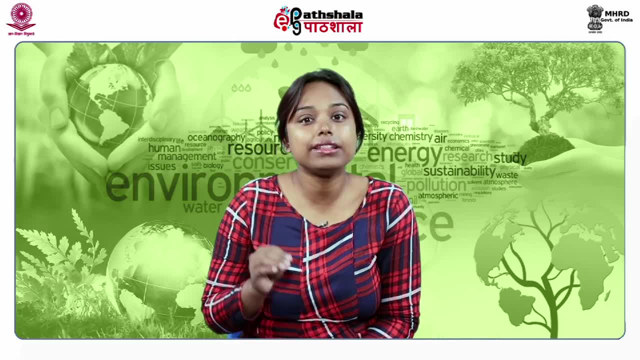 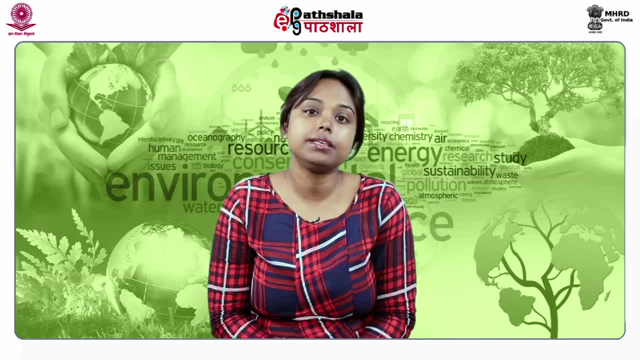 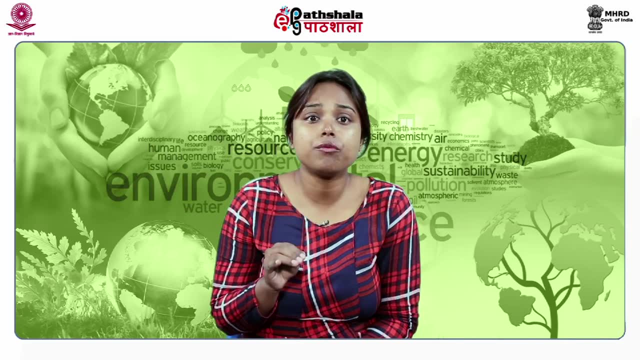 So the solution is absorbed by the resin, So the solution is absorbed by the resin. And finally, regenerating the resin by removing the absorbed chemicals, by simply washing with proper solvent. The adsorption of nonpolar molecule onto a hydrophobic resin results primarily from the 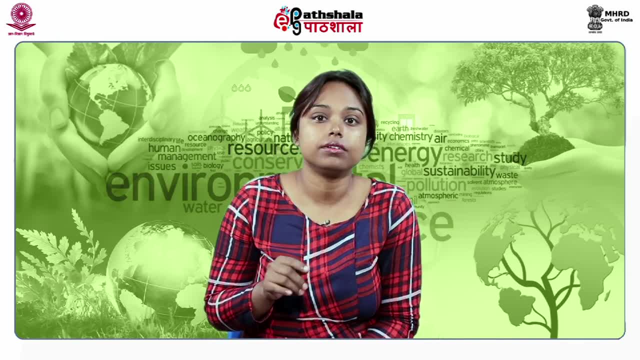 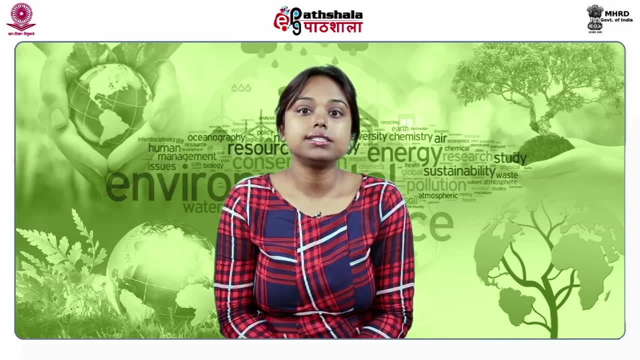 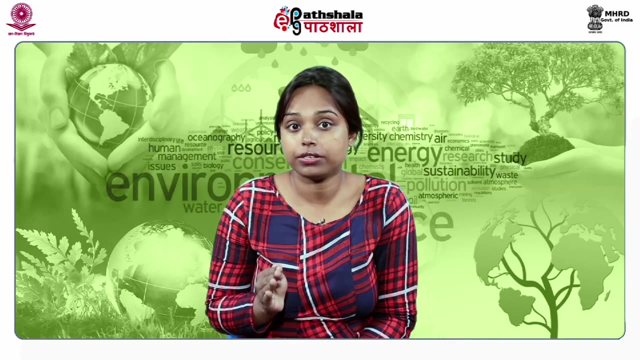 effect of van der Waals forces. In other cases, other types of interaction, such as dipole, dipole interaction and hydrogen bonding are important. In few cases ion exchange mechanism may be involved. For the removal of organic dye waste waste from wastewater, two different resins are employed, In this case the waste stream. 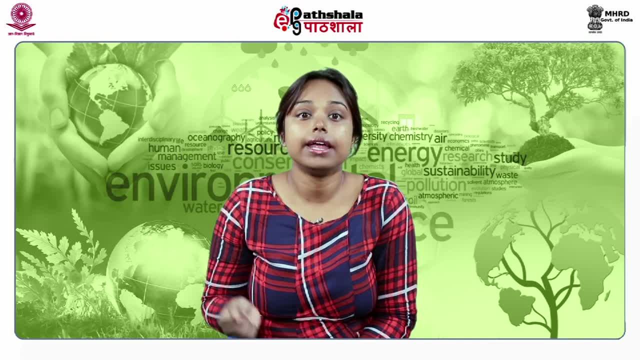 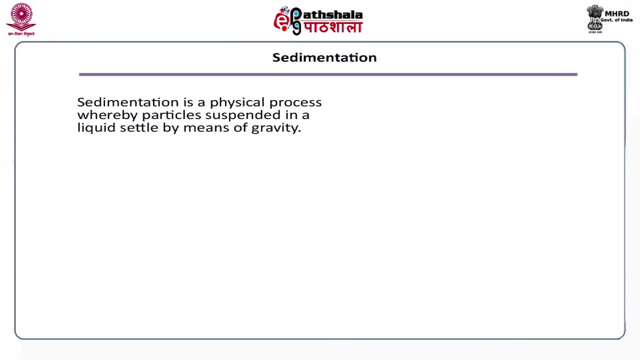 is first contacted with normal polymeric adsorbent and then with an ion exchange resin, Now sedimentation. Sedimentation is a physical process whereby a particle suspended in liquid settles by means of gravity. Sedimentation can be either a batch or continuous process. 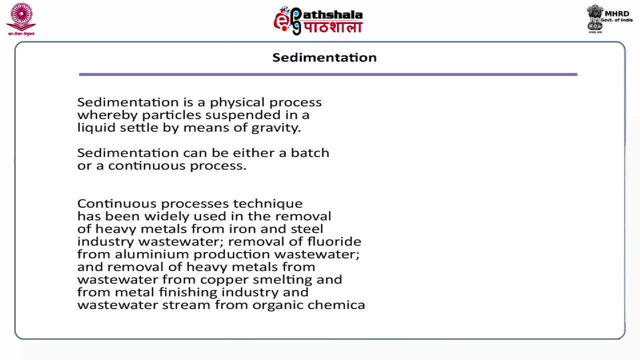 This process technique has been widely used in the removal of heavy metals from iron and steel industry wastewater, removal of fluoride from aluminium production wastewater and removal of heavy metals from wastewater from copper smelting and from metal finishing industry and wastewater stream from organic chemicals. A basin or container of sufficient size to 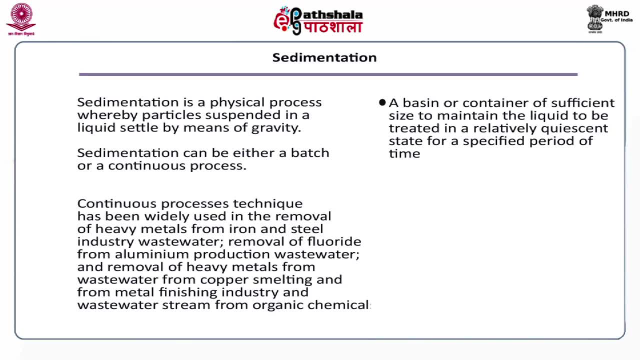 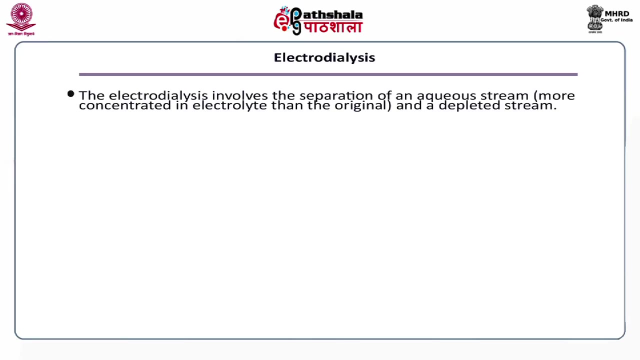 maintain the liquid to be treated in relatively quiescent state of a specified period of time. A means of directing the liquid to be treated into the above basin in a manner conducive to settling. A means of physically removing the settled particle from the liquid. Now next is electro dialysis. Electro dialysis involves the separation of an aqueous stream. 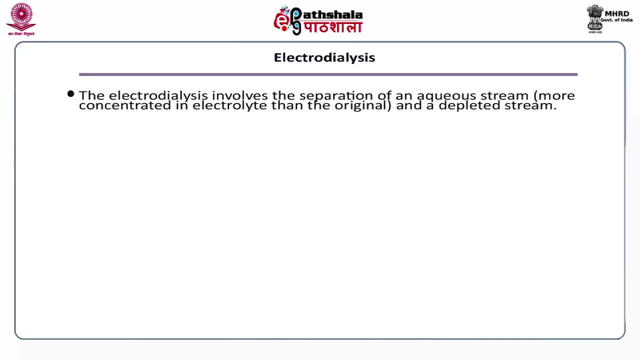 which is more concentrated in electrolyte than the original and a depleted stream. Success of the process depends on special synthetic membrane which is used to separate the liquid, usually based on ion exchange resin, which are permeable only to single type of ion. The feed water is passed through compartments formed by the space between alternating cation. 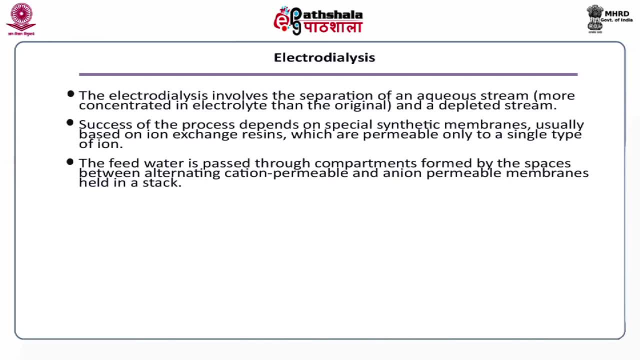 permeable and anion permeable membrane held in a stack. At each end of stack is an electrode having the same area as the membrane. A DC potential applied across the stack causes positive and negative ions to migrate in opposite directions. This technique has been used for 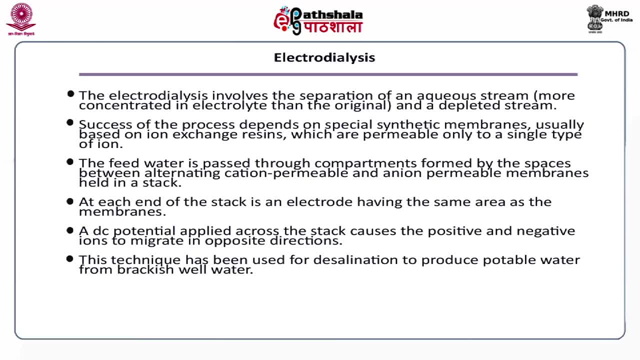 desalination to produce potable water from brackish well water. In food industry, electro dialysis is used for desalinating way. The chemical industry uses this technique for enriching or depleting solutions and for removing mineral constituent from product stream. 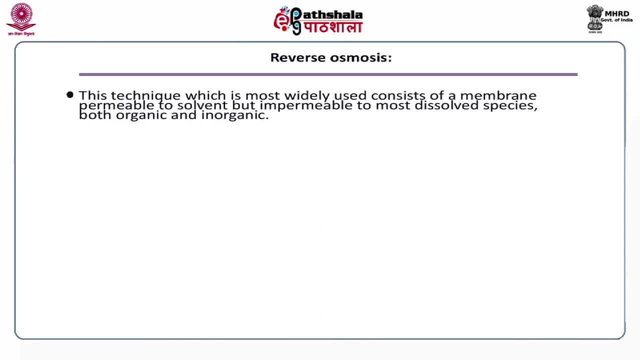 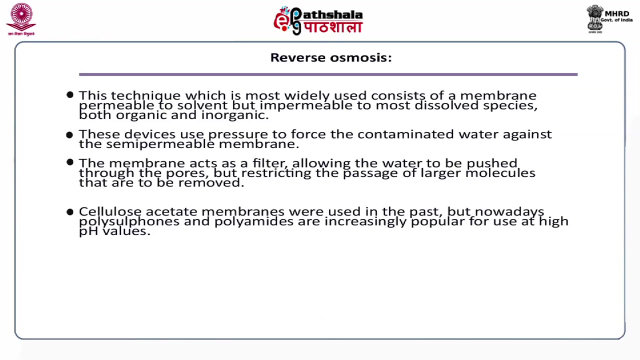 Now next is reverse osmosis. This technique, which is most widely used, consists of a membrane permeable to solvent. This membrane is impregnated with nicotine when activated, which is the solution of nucleic acid. Hide wasn't used in the same way. 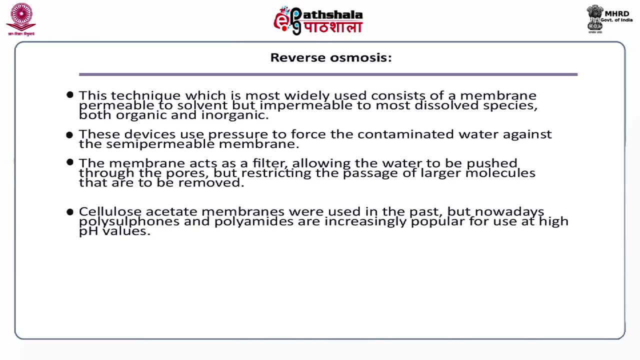 But a direct dose of Jeremy vitamin are increasingly popular for use at high pH values. Because of the susceptibility of membrane to chemical attack and fouling and the susceptibility of the flow system to plugging and erosion, it is commonly to reprocess the feed water to remove oxidizing material. 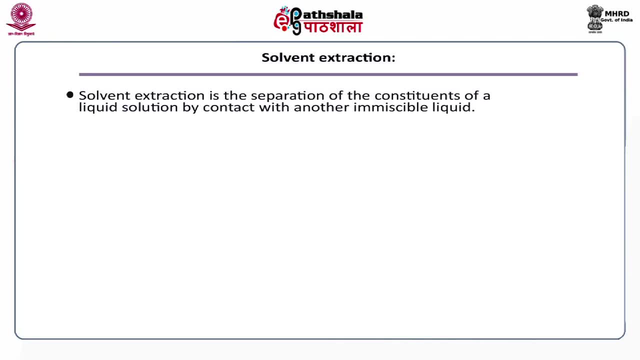 Now next is solvent extraction. Solvent extraction is the separation of constituent of liquid solution by contact with another immiscible liquid. If the substance comprising the original solution distribute themselves differently between the two liquid phases, a certain degree of separation will result, and this may be enhanced by the use of multiple contacts. 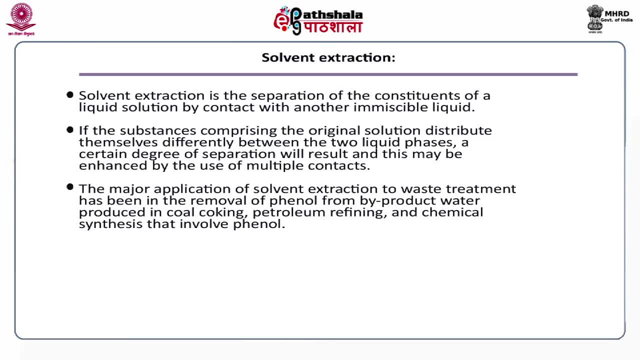 The major application of solvent extraction to wastewater treatment has been in: the removal of phenol from by-product water produced in coal, caulking, petroleum refining and chemical synthesis that involve phenol. The use of supercritical fluids, SCF, most commonly CO2, as extraction solvent. 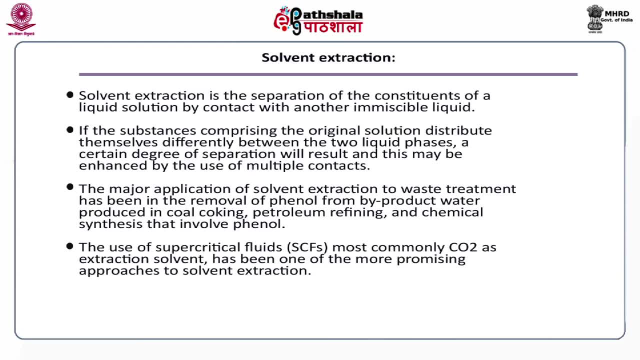 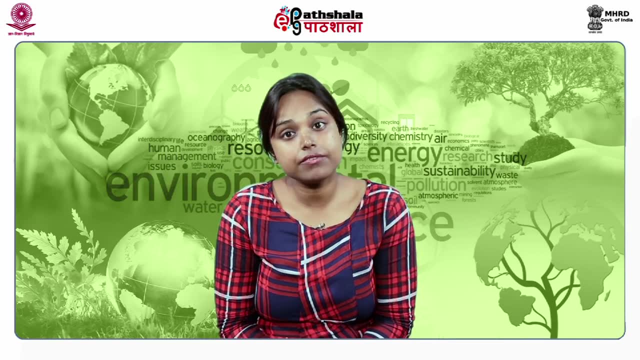 has been one of the most promising approach to solvent extraction. SCF are fluid existing at or above lowest temperature at which condensation may occur. Now next is desalination. Desalination is expensive. Desalination is expensive And energy intensive and can probably be justified only in cases. 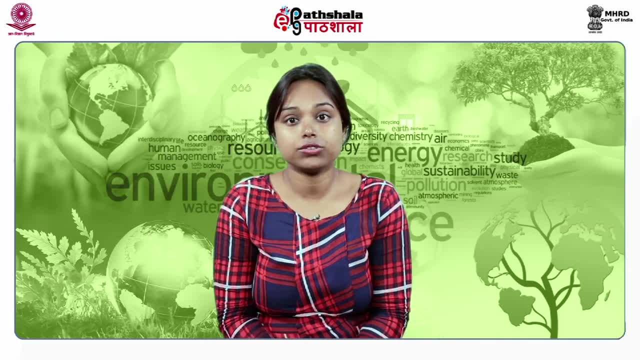 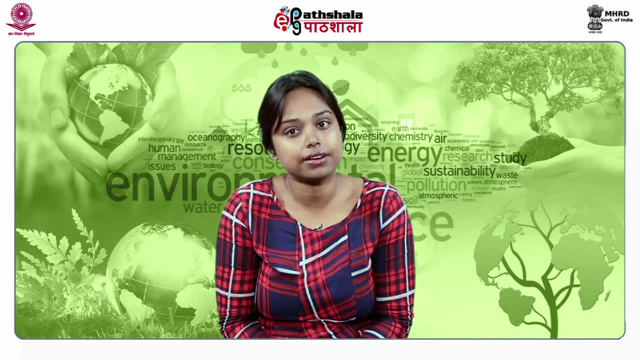 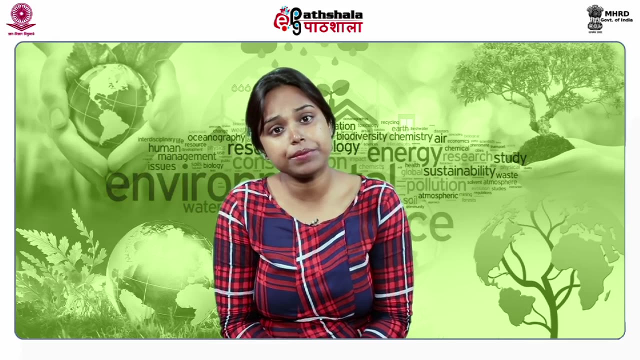 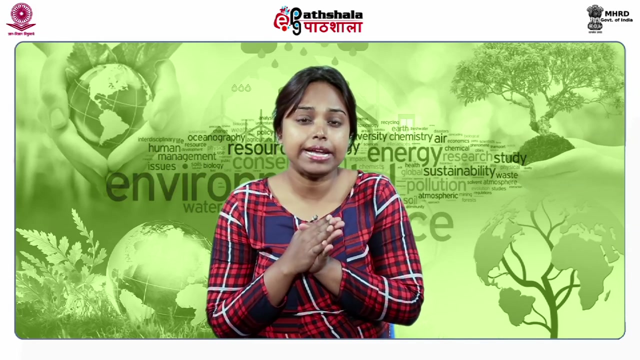 where valuable product recovery is feasible. like solvent recovery, This technique has only limited application in the treatment of diluted aqueous hazardous waste. Now next is evaporation. Evaporation process is used for the treatment of hazardous waste such as radioactive liquids and sludges, and concentrating of plating and paint solvent. 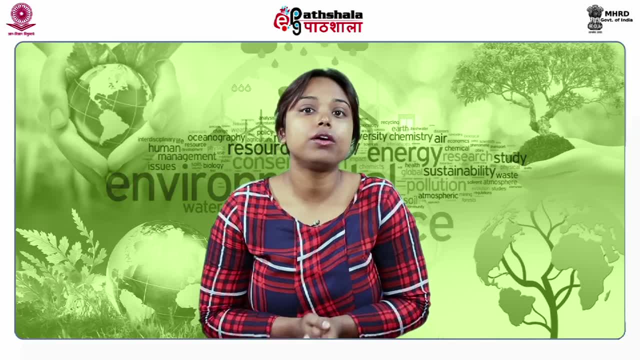 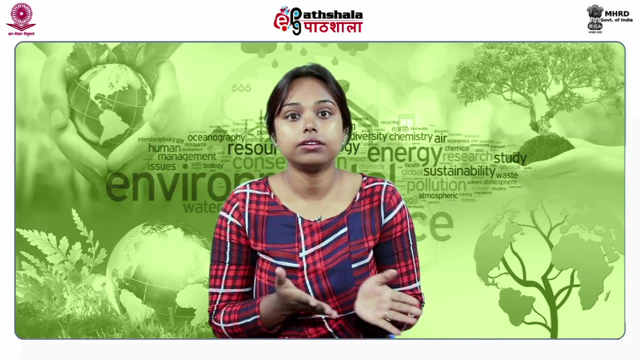 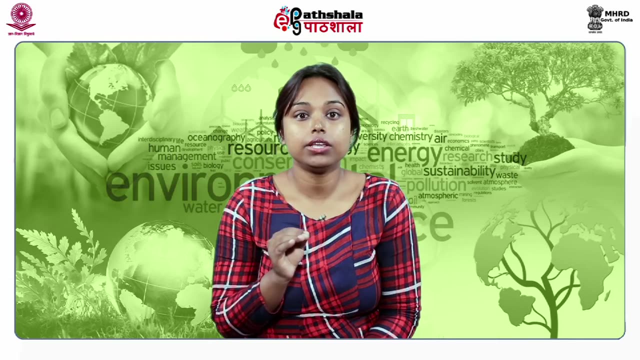 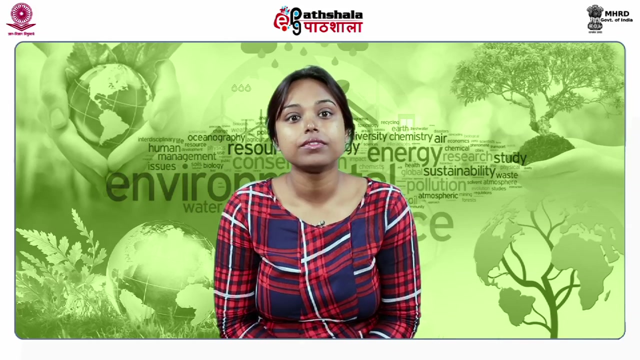 waste. among many other applications, It is capable of handling liquids, slurries and sometimes sludges, both organic and inorganic, containing suspended or dissolved solids or dissolved liquids. Where one of the compound is essentially non-volatile, It can be used to reduce waste volume prior to landfill disposal or incineration. 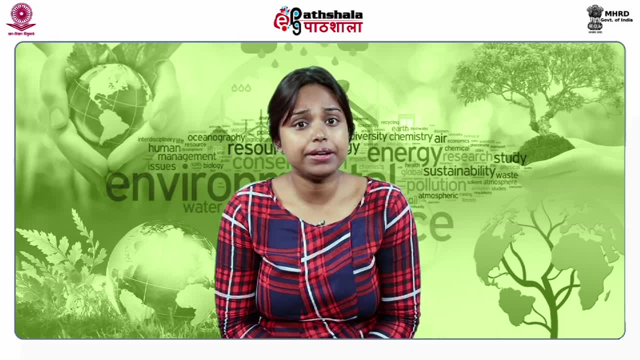 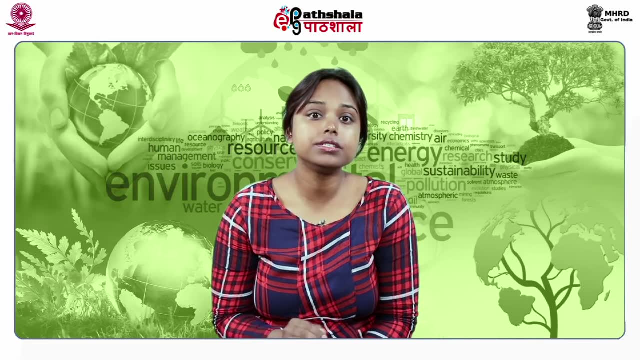 The major disadvantage of evaporation and high capital and operating cost and high cost of waste is that it is not a primary treatment process and high energy requirement. This process is more adaptable to waste waters with high concentration of pollutants. Now next is filtration. 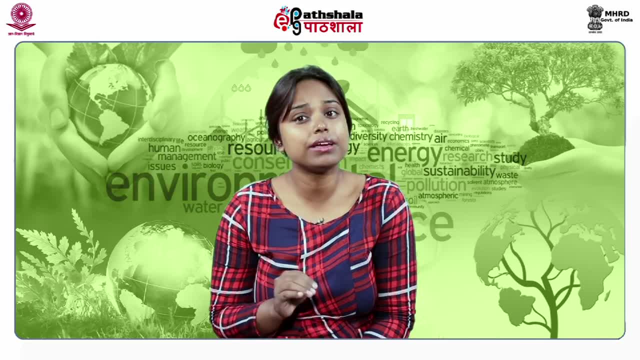 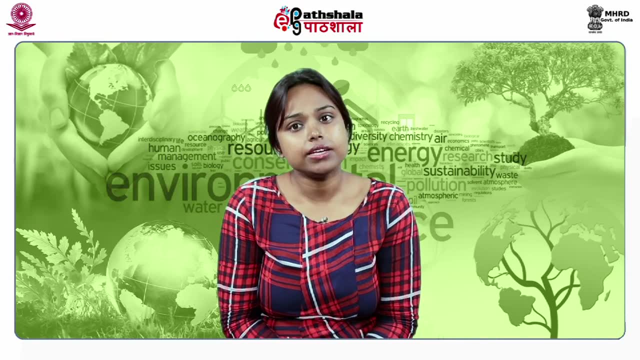 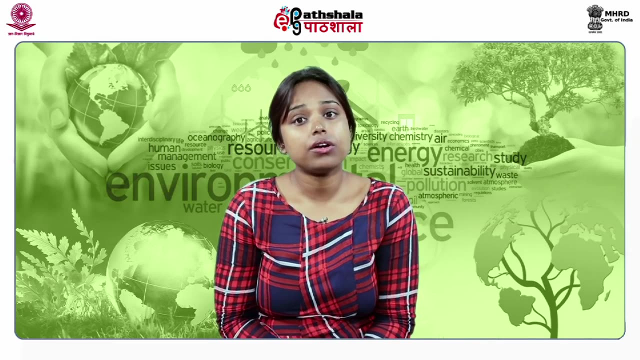 Filtration is well developed, economical process used in full scale treatment of many industrial waste waters and waste sludges. Energy requirements are relatively low and operational parameters are well defined. However, it is not a primary treatment process and is often used for the treatment of waste. 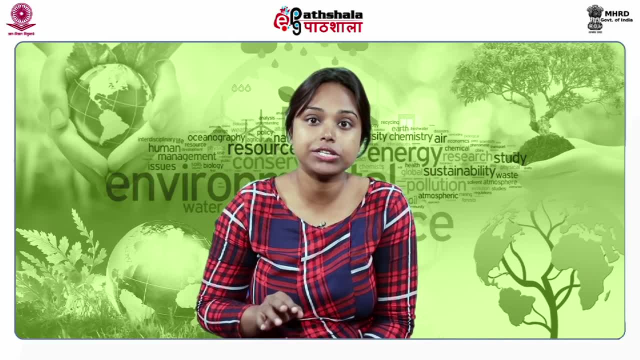 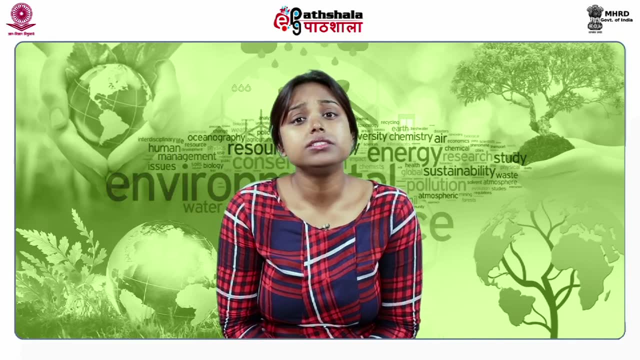 It is often used in conjunction with precipitation, flocculation and sedimentation to remove these solids. Now next is flocculation. Chemicals used for flocculation include alum, lime, ferric chloride, ferrous sulphate and polyelectrolytes. 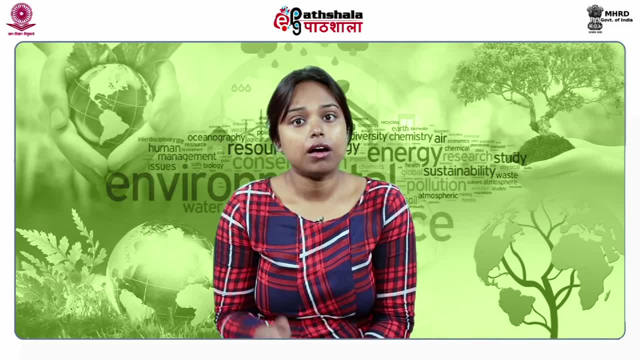 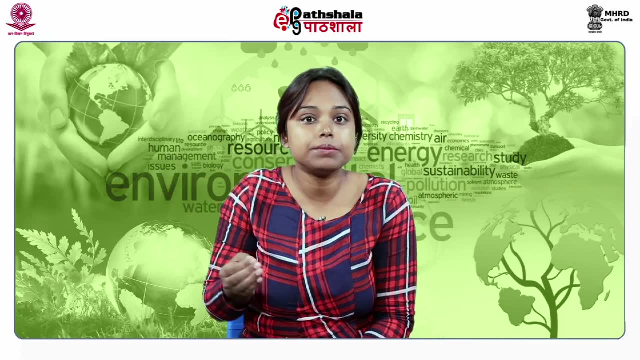 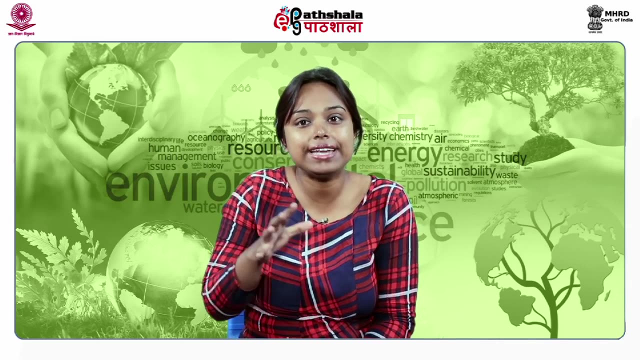 The inorganic flocculants, such as alum, upon mixing with water. the slightly higher pH of water causes them to hydrolyze to form gelatinous precipitates of aluminium hydroxide. It is partially because of their large surface area they are able to entangle small particles and thereby create larger particles. 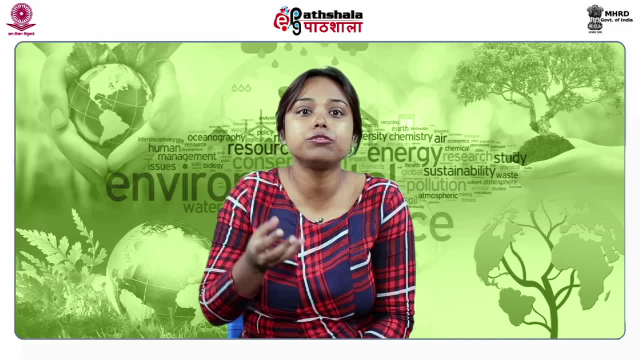 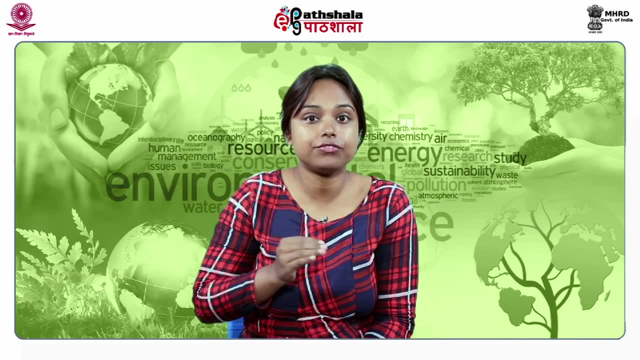 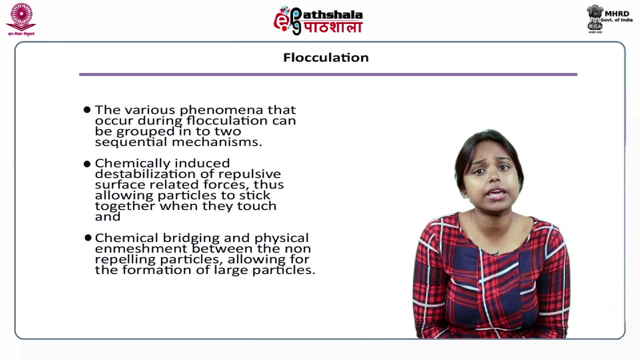 Once suspended particles have been flocculated into larger particles, they usually can be removed from the liquid by sedimentation, Provided that a sufficient density difference exists between suspended matter and the liquid. The various phenomena that occur during flocculation can be grouped into two sequential mechanisms. Chemically induced destabilization of repulsive surface related forces, thus allowing particle to stick together when they touch, and chemical bridging and physical enmeshment between the non-repelling particle, allowing for the formation of large particles. Now chemical treatment methods. Under chemical treatment methods, first is chemical oxidation and reduction. 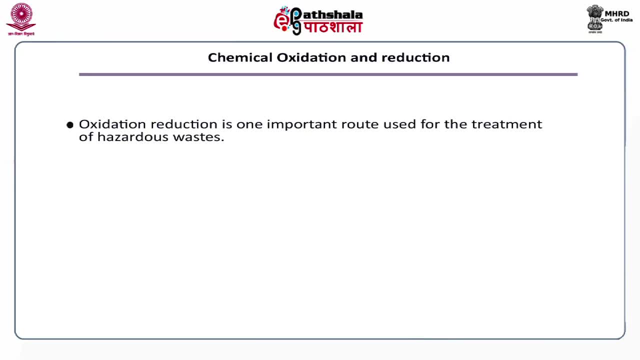 Oxidation reduction is the process of chemical oxidation and reduction. Oxidation reduction is one of the important route used for the treatment of hazardous waste. It is process by which hazardous waste are converted into a form that shows reduced or no toxicity, reduced or no mobility and remains inert. 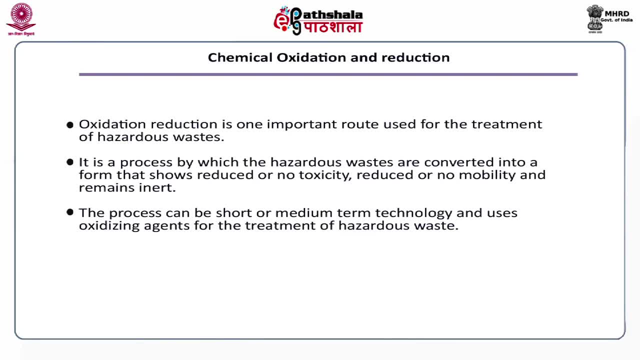 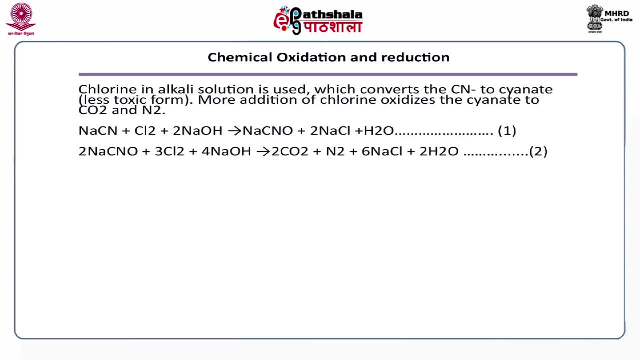 The process can be short or medium term. technology and use. oxidizing agent for the treatment of hazardous waste, Chlorine in alkali solution is used, which converts cyanide into cyanide, Which is lesser toxic form. More addition of chlorine oxidizes the cyanide to carbon dioxide and nitrogen gas. 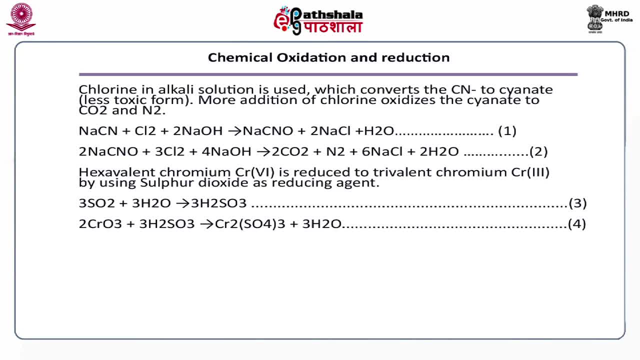 Hexavalent chromium is reduced to trivalent chromium by using sulphur dioxide as a reducing agent, Which is shown in the reaction below. Then, in another example, iron is oxidized and precipitated as ferric oxide, which is mentioned below. Then sulphur dioxide is oxidized to sulphuric acid. 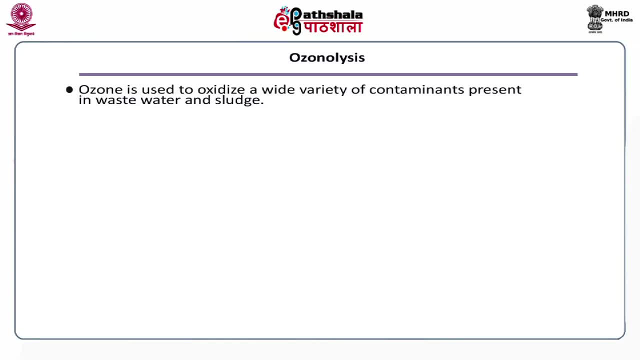 Now, moving on to ozonolysis. Ozone is used to oxidize a wide variety of contaminants present in waste water and sludge. Ozone is generated by an electrical discharge through dry air or oxygen. Ozone is also used to destruct TCDD and PCBs. 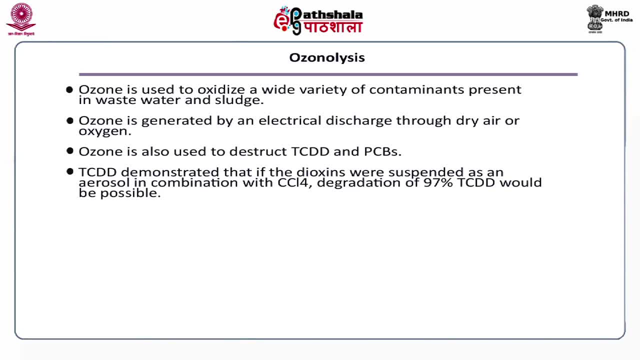 TCDD demonstrated that if the dioxins were suspended as an aerosol in combination with CC14, degradation of 97% TCDD would be possible. Destruction of polychlorinated phenols and pesticides by ozone can be done in conjunction with UV radiation. 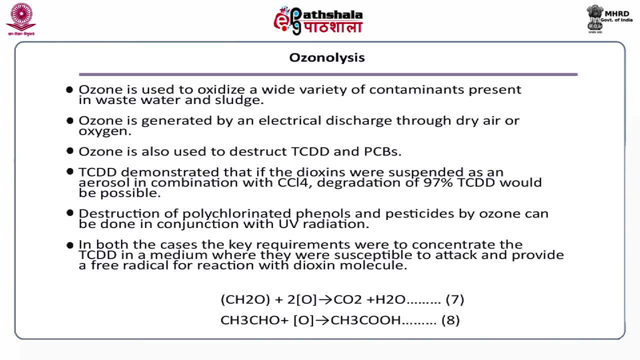 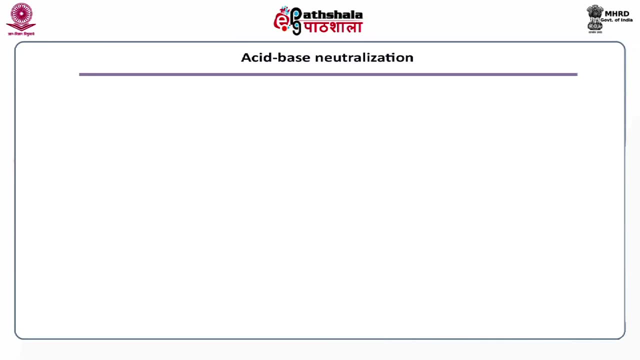 In both the cases, the key requirement were to concentrate the TCDD in a medium where they were susceptible to attack and provide a free radical for reaction with dioxin molecules. The reactions are mentioned below Now. next is acid based neutralization. 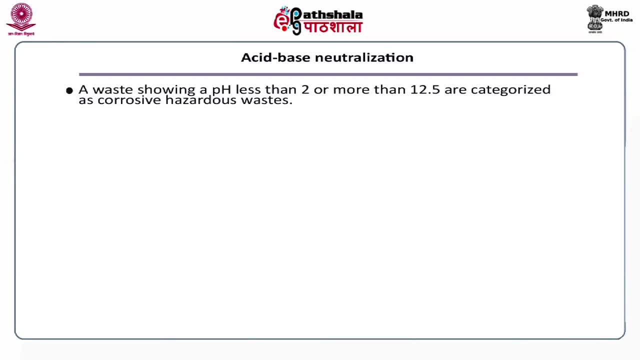 A waste showing a pH less than 2 or more than 12.5 are characterized as corrosive, hazardous waste. They can be neutralized by acid based reactions. Lime is used to neutralize acid waste. Addition of slaked lime to acidic waste in a continuously stirred chemical reactor. 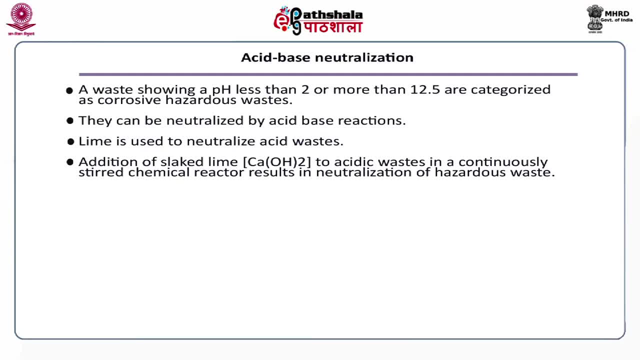 results in neutralization of hazardous waste Similar to lime, sulfuric acid and acetic acid is used for neutralizing alkaline waste. Certain alkaline wastes are also neutralized by bubbling gaseous CO2, forming carbonic acids. In addition to this, may other waste treatment process require prior pH adjustment. 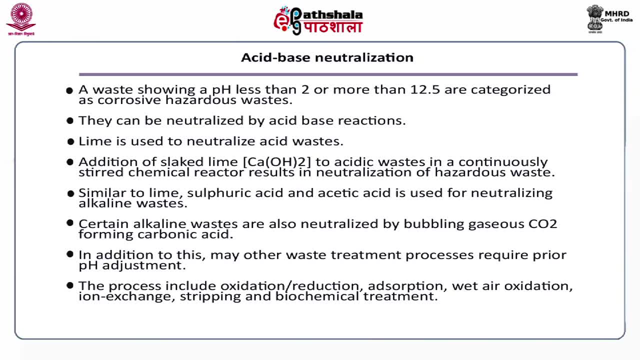 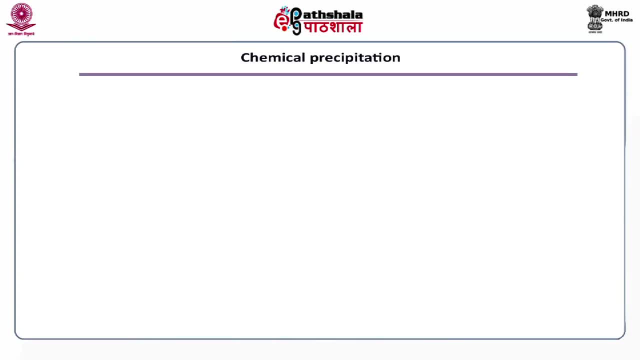 The process include oxidation reduction, adsorption, wet air oxidation, ion exchange, stripping and biochemical treatment. Now, next is chemical precipitation. Precipitation is applicable for mixed waste that contain both organic and inorganic species. By this method, the toxic substance or metals are precipitated using chemicals. 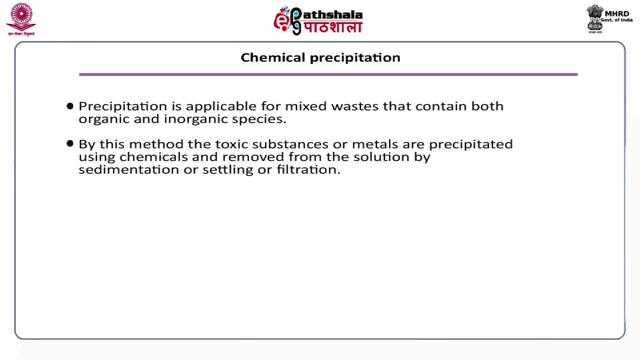 and removed from the solution by sedimentation, settling or filtration. Alteration of solution pH will minimize the solubilization of heavy metals, which can further be precipitated as precipitable hazardous constituents. Slaked lime or caustic soda is used for precipitation of metal ions as metal hydroxides. 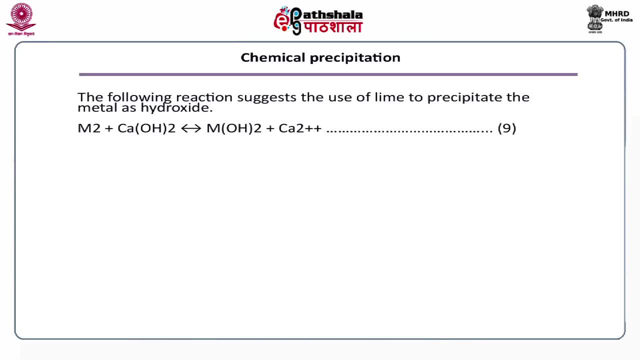 Now the following reaction suggests the use of lime to precipitate the metal as hydroxides. Chromium is precipitated as hydroxide. Sodium carbonate is also used to precipitate metals as hydroxides, Carbonates, basic carbonate salts and etc. 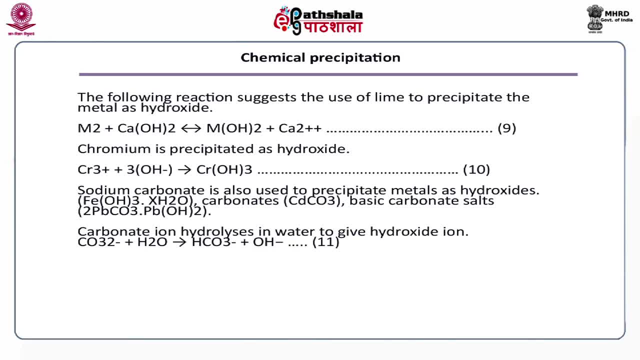 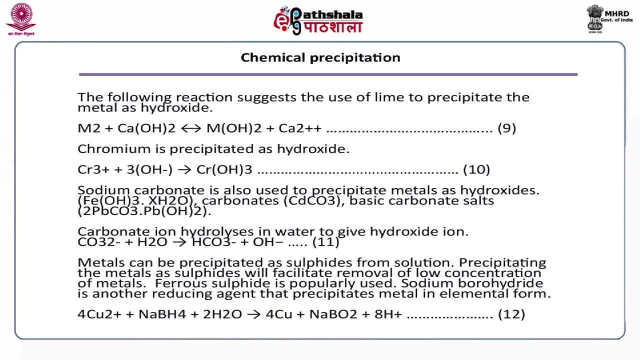 Carbonate ion hydrolysis in water to give hydroxide ions. Metals can be precipitated as sulphides from solution. Precipitating the metal as sulphides will facilitate removal of low concentration of metals. Ferrous sulphide is popularly used. 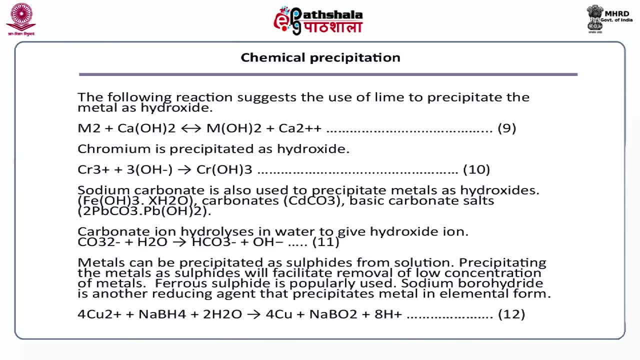 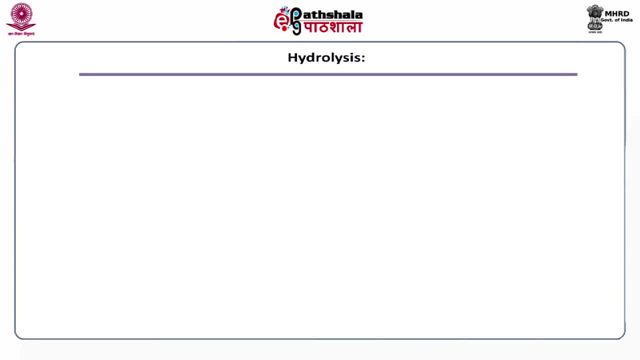 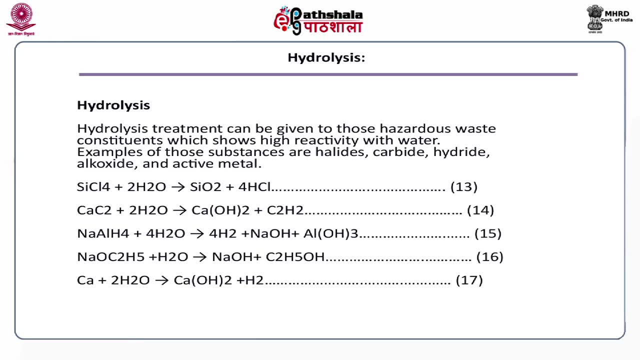 Sodium borohydride is another reducing agent that precipitates metal in elementary particles In elemental form. the reaction is given below Now. next is hydrolysis. Hydrolysis treatment can be given to those hazardous waste constituents which show high reactivity with water. 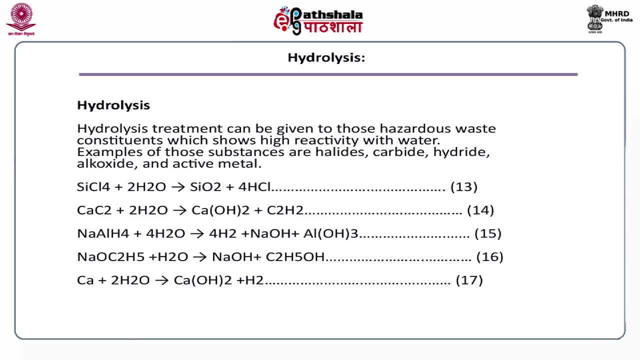 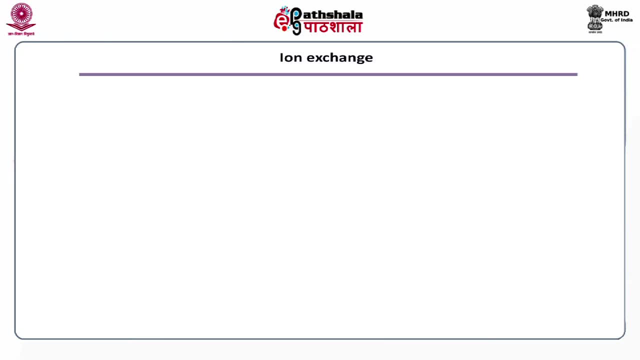 Example of those substances are halides, carbide hydride, alkoxide and active metals. Next is ion exchange. Ion exchange is best suited for waste that have undergone pre-treatment or minimum treatment with other chemical and physical methods. It is suitable for removing inorganic chemical species that are in dissolved form. 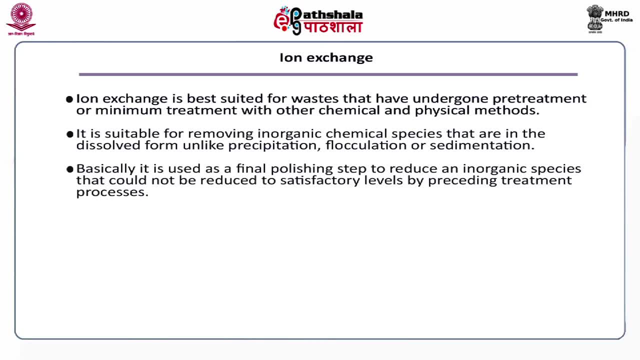 unlike precipitation, flocculation or sedimentation. Basically it is used as final polishing step to reduce inorganic species that could be reduced to satisfactory level by preceding treatment process. Nickel, cyanide, complex and chromate ion From hazardous waste solution are removed by anion exchange membranes. 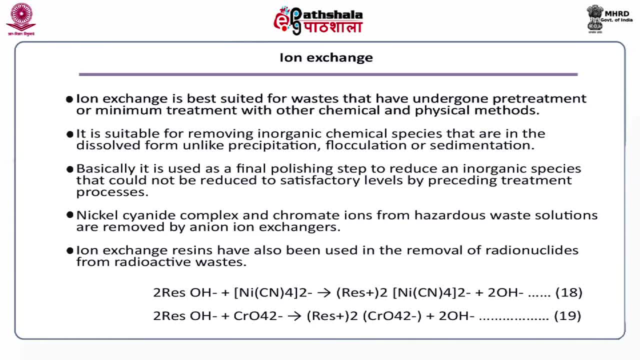 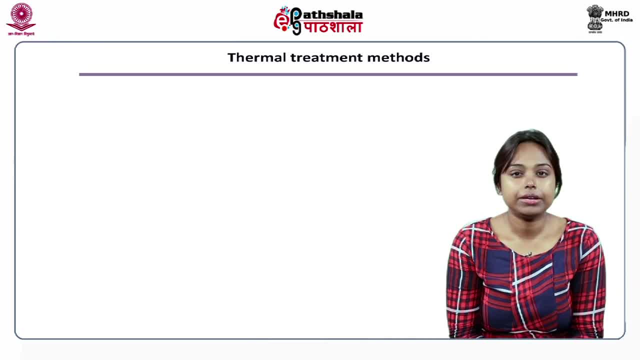 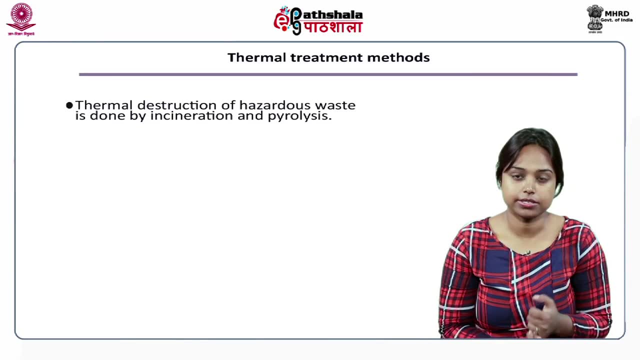 Ion exchange resins have also been used in removal of radionuclides from radioactive waste. Now, thermal treatment methods- Thermal destruction of hazardous waste- is done by incineration and pyrolysis. Incineration is a process that combusts the waste at high temperature. 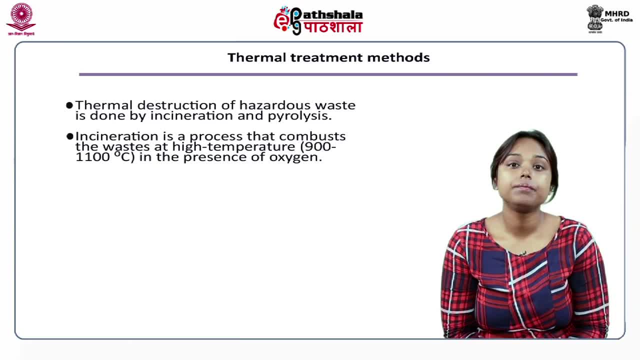 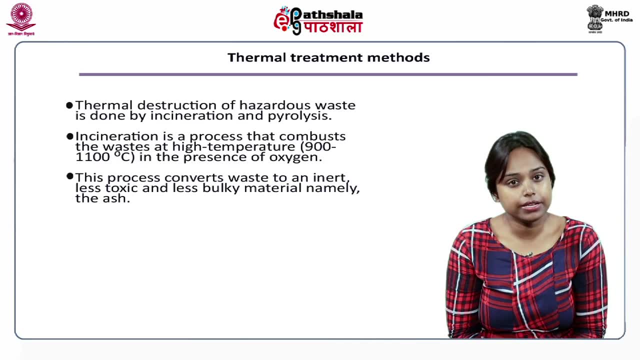 ranging between 900 to 1100 degree Celsius. in the presence of oxygen, This process converts waste to an inert, less toxic and less bulky material, namely ash. The organic elements, such as carbon hydrogen and oxygen, are converted wholly or partially to gaseous form. 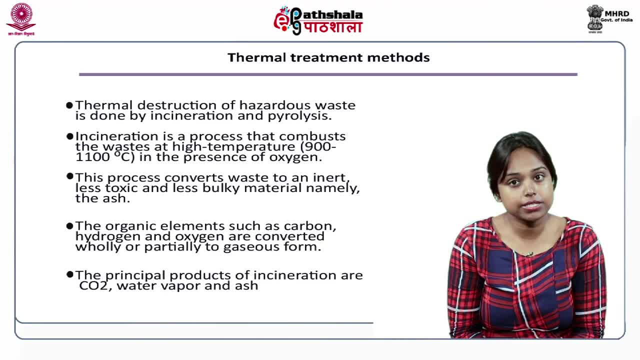 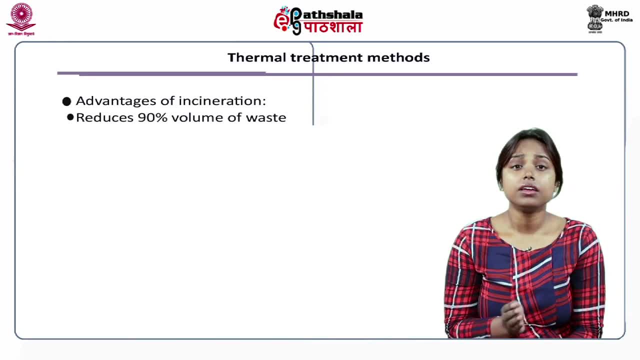 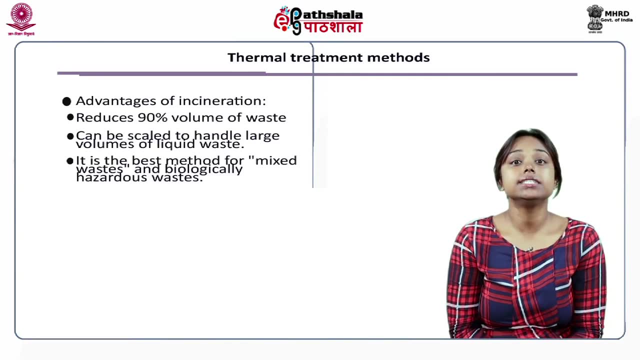 The principal products of incineration are carbon dioxide, water, vapour and ash. Now let us see the advantages of incineration: Reduces 90% volume of waste. Can be scaled to handle large volumes of liquid waste. It is the best method for mixed waste and biologically hazardous waste. 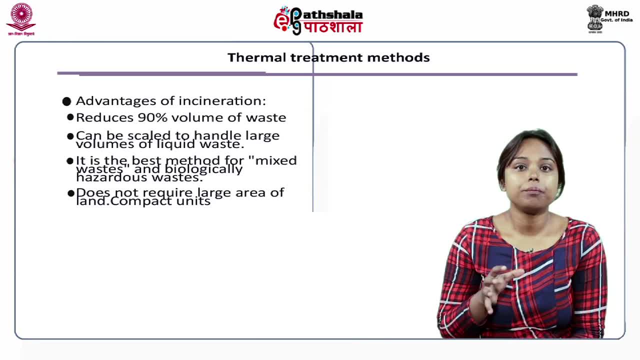 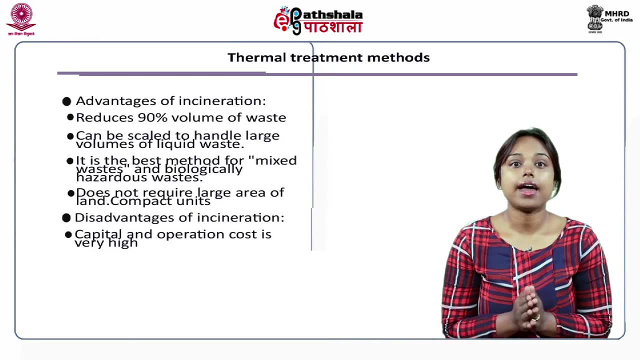 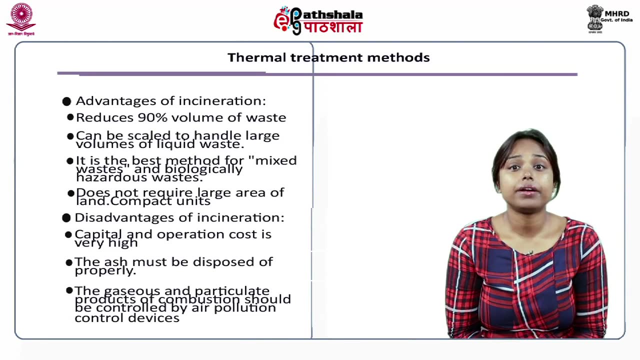 It does not require large area of land: compact units. Now we will see disadvantages of incineration. It has high capital and operation cost. The ash must be disposed of properly. The gaseous and particulate products of combustion should be controlled by air pollution control devices. 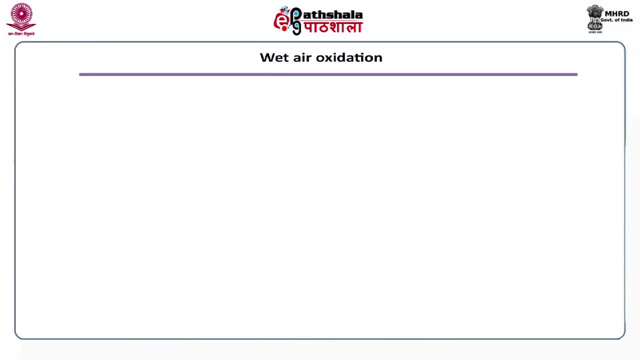 Now next is wet air oxidation. Wet air oxidation is the process by which dissolved or suspended organic substance are oxidized in aqueous phase at temperature and pressure of 150 to 3000 and to 50 degree Celsius and 2000 kilopascals. 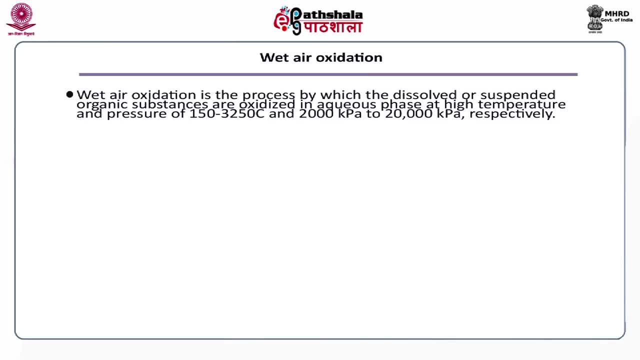 To 20,000 kilopascals respectively. Water acts as catalyzing agent and moderator by removing excess heat in reaction mixture. Water also acts as an excellent heat transfer medium, so that the wet air oxidation process becomes thermally substance staining at low organic feed conditions. 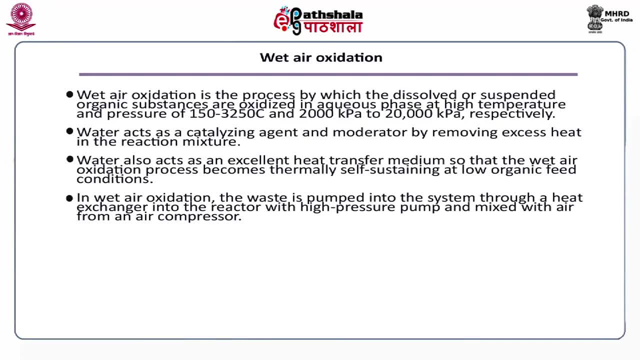 In wet air oxidation. the waste is pumped into the system through heat exchanger, Into the reactor with high pressure pump and mixed with air from air compressor. High pressure facilitates dissolving of oxygen in water. Within the reactor, the organic waste is reacted with atmospheric oxygen. 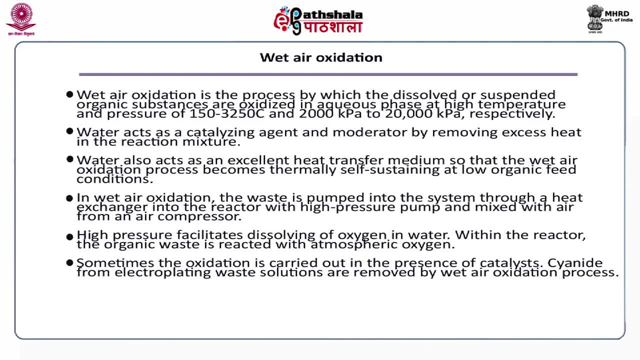 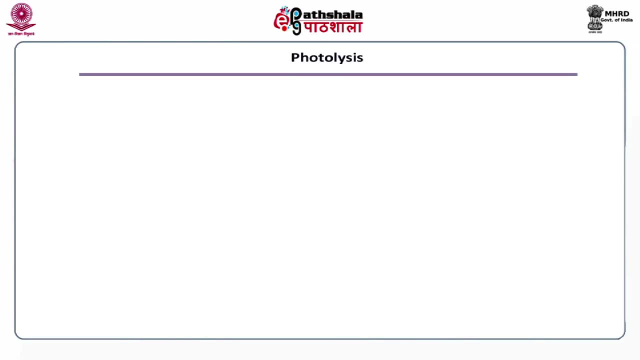 Sometimes the oxidation is carried out in presence of catalyst Cyanide from electroplating waste solution, removed by wet air oxidation process. The process can be used for removal of different metals. Now, photolysis. In photolysis, light is used as an agent to cleave chemical bonds of hazardous waste materials. 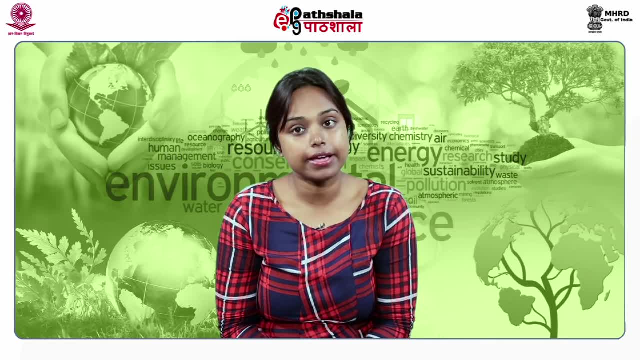 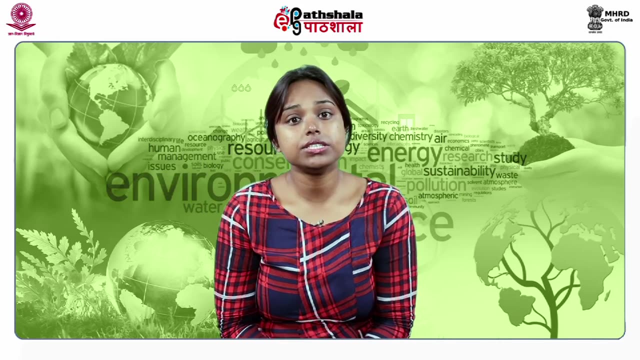 Initially, the chemical species is excited by light. It is usually a di-radical state, because di-radical possess sufficient energy to undergo chemical reaction. The success or effectiveness of the process depends on chemical structure of the compound, Efficiency of the radiation source and medium in which the reaction is carried out. 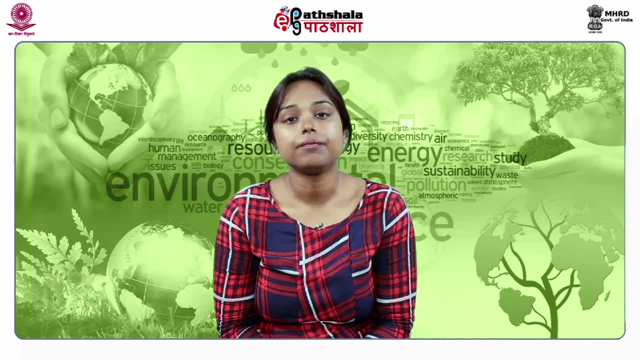 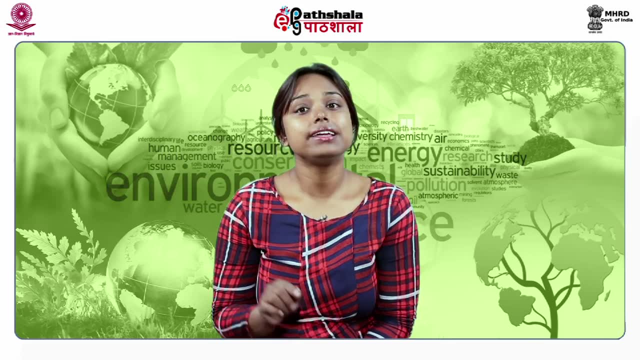 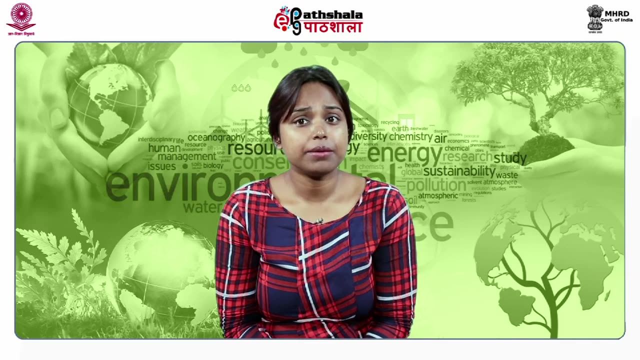 The end product also determines the efficiency of the process. Polychlorinated biphenyls and chlorinated dibenzopedioxins are destroyed by photolysis. The three requirements of photolysis of tetrachlorodibenzopedioxins are: 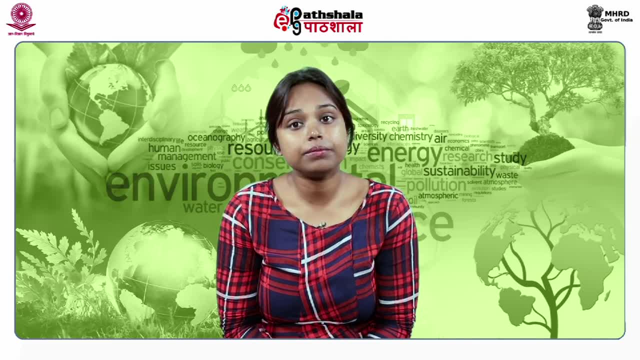 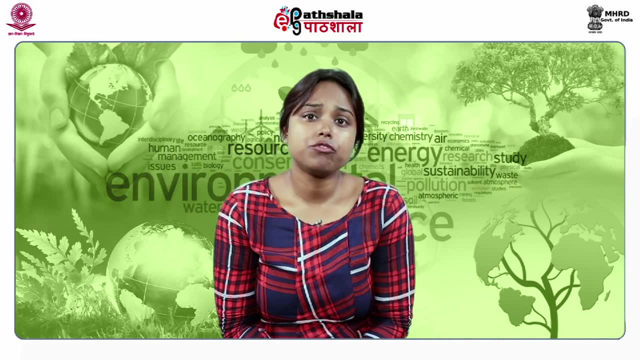 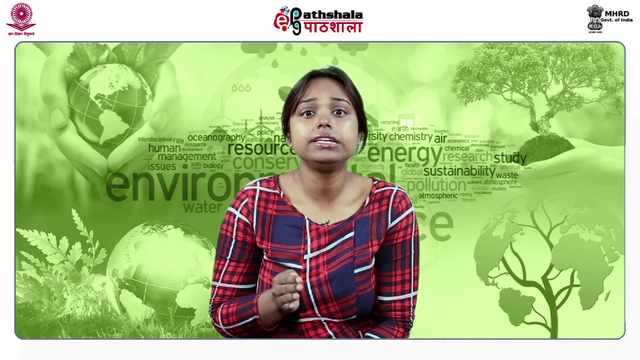 1. Dissolution in light transmitting film. 2. Presence of organic hydrogen order. 3. UV light. Generally, during photolysis reaction HO radical is formed, which play an important role in chain reactions Resulting in destruction of the compound. 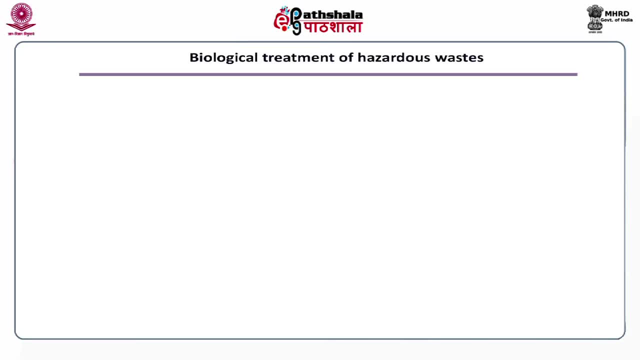 Now third one is biological treatment of hazardous waste. Biological process are simple, cost-effective and eco-friendly process. However, its application to hazardous waste is slightly limited due to its toxic nature, which is harmful to biological agents. The biodegradability of the waste depends on physical and chemical properties of the compound. 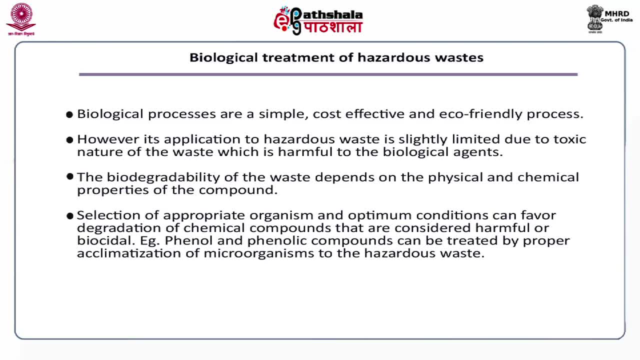 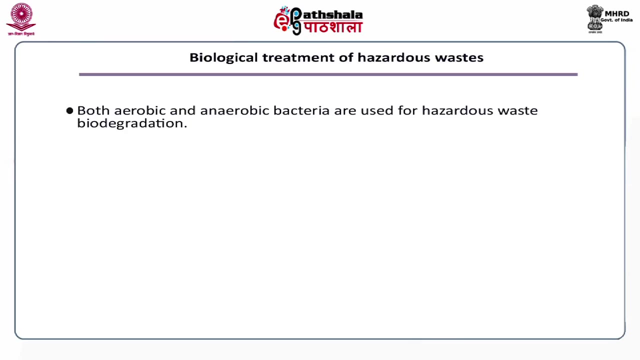 Selection of appropriate organisms and optimum condition can favor degradation of chemical compounds that are considered harmful or biocidal. Example: phenol and phenolic compounds can be treated by proper acclimatization of microorganisms to the hazardous waste. Both aerobic and anaerobic bacteria are used for hazardous waste biodegradation. 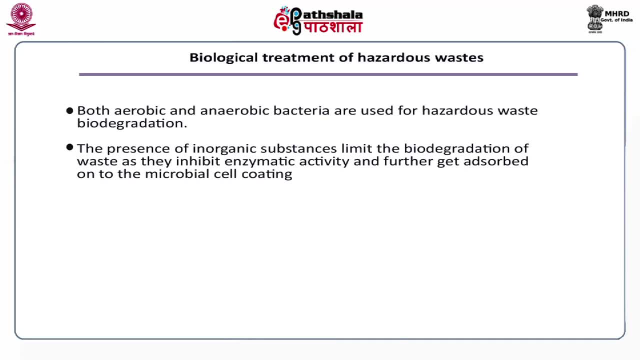 The presence of inorganic substance limit the biodegradation of waste, as they inhibit enzymatic activity and further get adsorbed onto the microbial cell coating. Landfill leachate is treated with microorganisms. During the process, H2S is generated, which precipitates toxic heavy metals. 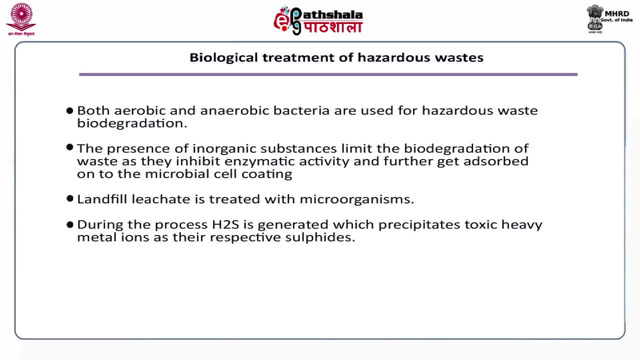 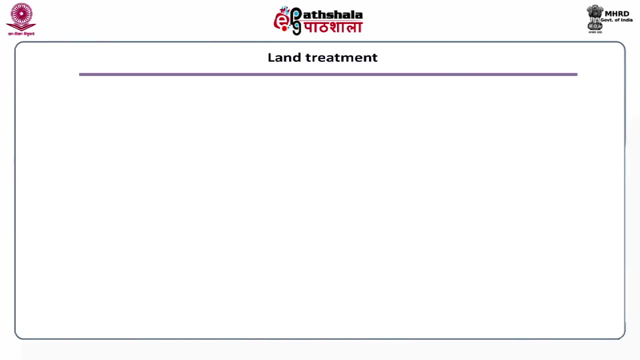 This precipitates toxic heavy metal ions to their respective sulfides. The overall degradation of hypothetical organic compound can be written as follows, in which we can see: the end product of degradation is carbon dioxide and water. Now next is land treatment. The application of waste to solid surface in a controlled manner is termed as land treatment of hazardous waste. 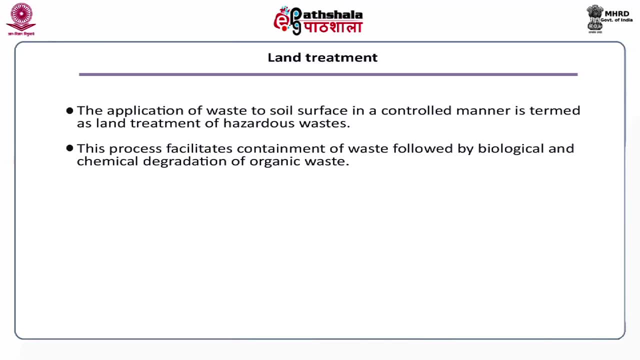 This process facilitates containment of waste, followed by biological and chemical degradation of organic waste. This type of treatment is different from landfilling. Here, the soil is used to detoxify, immobilize and degrade all or portion of applied waste. Landfills contain waste and control its migration from the site. 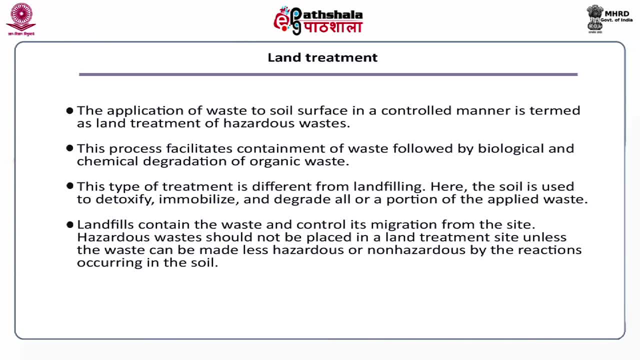 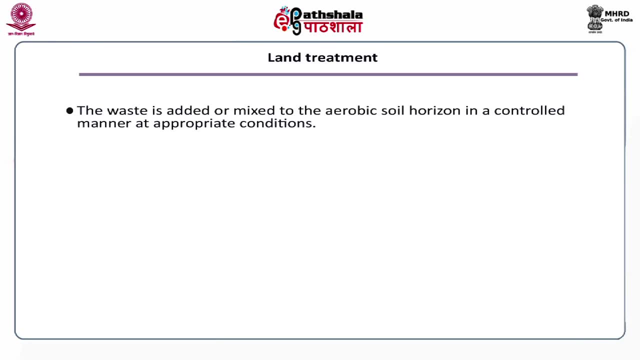 Hazardous waste should not be placed in a land treatment site unless the waste can be made less hazardous or non-hazardous by reaction occurring in the soil. The waste is added or mixed to aerobic soil horizon in a controlled manner at appropriate conditions. By this process, the physical, chemical and biological characteristics of waste are altered. 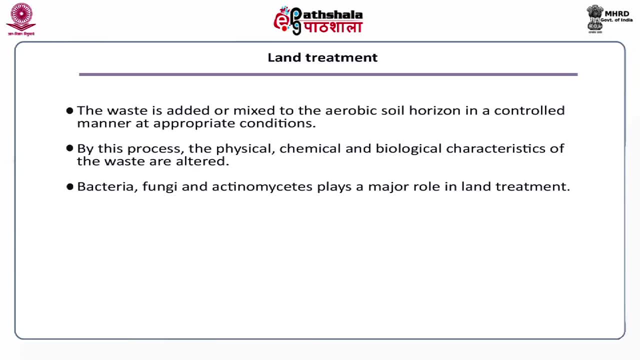 Bacteria, fungi and actinomycetes play a major role in land treatment. Genus Agrobacterium, Anthrobacterium, Bacillus, flavobacterium, Pseudomonas are some of the bacteria involved in the degradation. 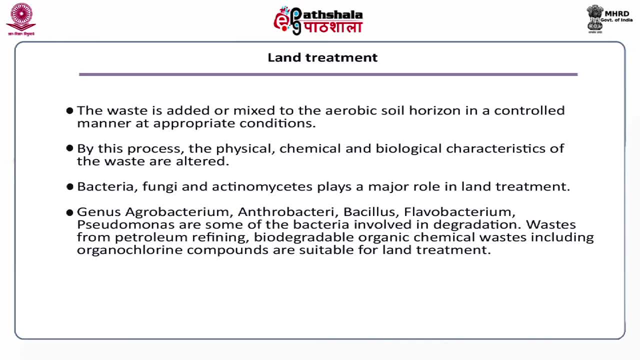 Waste from petroleum refining. biodegradable organic chemical waste, including organochlorine compounds, are suitable for land treatment. Land treatment should not be applied to waste containing acids, bases, toxic inorganic compounds, salts, heavy metals and excessively soluble volatile compounds. 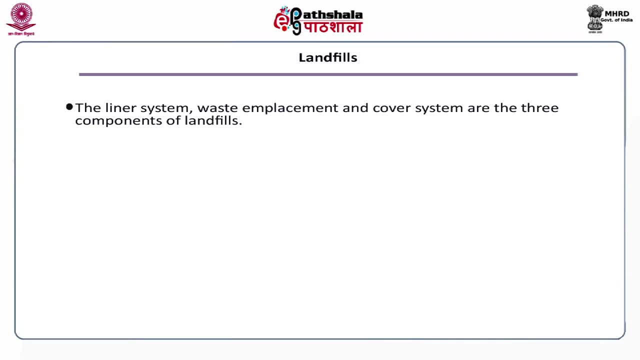 Last. Land Fills. The liner system, waste emplacement and cover system are the three components of land fills. Liners should be impermeable and avoid the contact between waste and surrounding environment. Leachate collection system, drain and leak detectors: two forms an integral part of landfills system. 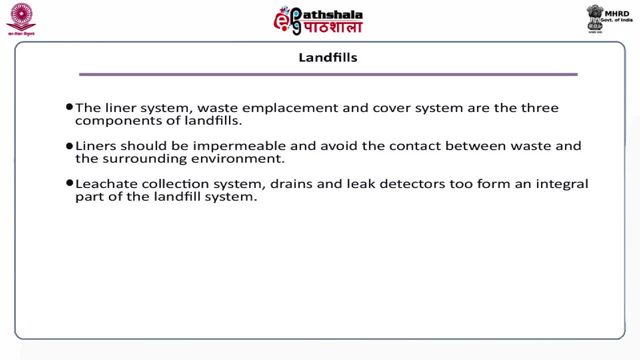 They ensure that leachate does not leave the disposal site. Hazardous wastes are contained in the waste collection system and it is seen as a very valuable part of the disposal site: Land Fills. The basics of the land filling system are 1.. 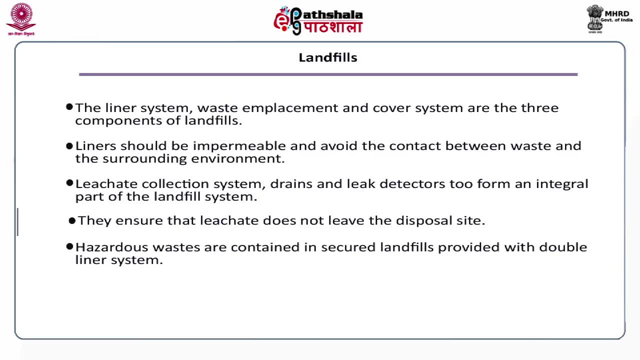 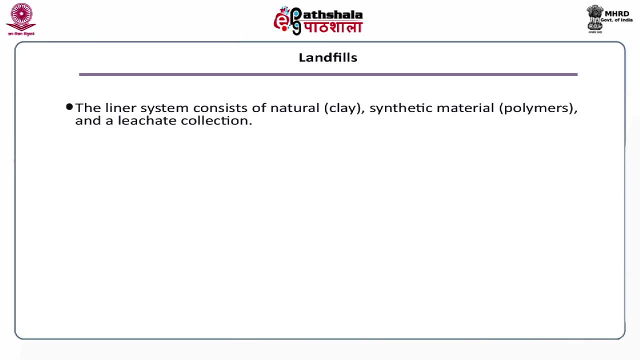 in secured landfills provided with double liner system. The liner system consists of natural clay, synthetic material such as polymer, and leachate collection. The primary barrier is synthetic polymer flexible membrane with separation layer of a thin geotextile or polymeric material such as SDPE, LDPE, PVC, etc. Now secondary barrier. Secondary barrier is: 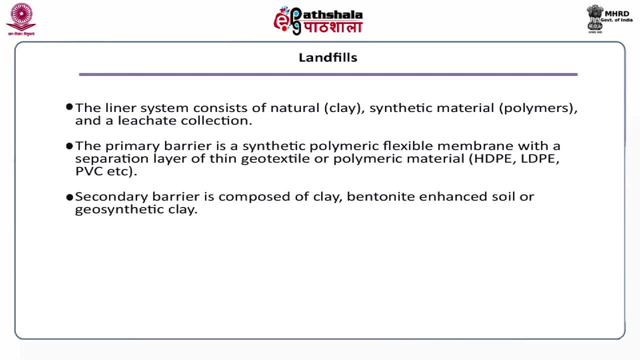 composed of clay, bentonite, enhanced soil or geosynthetic clay. A leachate collection tubes are layered between the waste and the protection layer. It channelizes the leachate to a pumping station, where they are removed and taken up for further treatment. An intermediate. 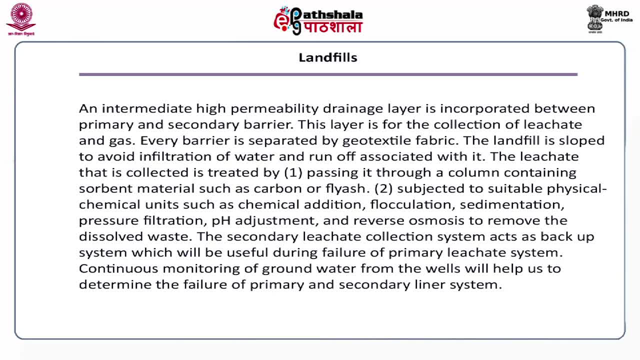 high permeability. drainage layer is incorporated between primary and secondary barrier. This layer is for the collection of leachate and gas. Every barrier is separated by geotextile fabric. The landfill is sloped to avoid infiltration of water and runoff associated with it. The leachate that is collected is treated by first passing it. 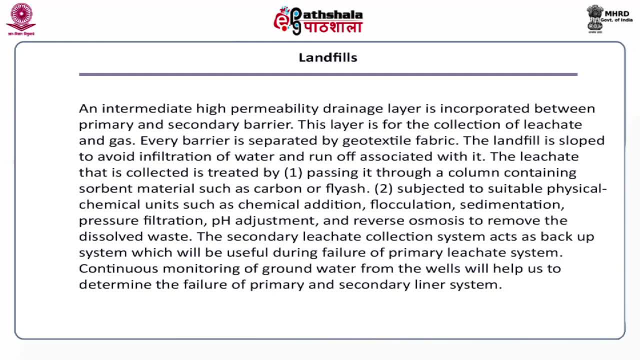 through a column containing sorbate material such as carbon or fly ash, Second, subjected to suitable physical chemical unit, such as chemical addition, flocculation, sedimentation, pressure treatment and reverse osmosis to remove the dissolved water. The secondary leachate collection system acts as a backup system which will be useful during. 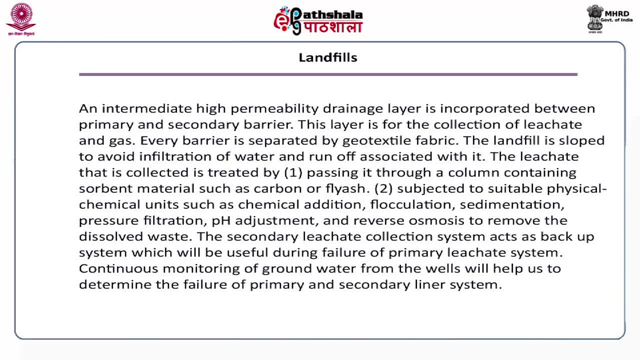 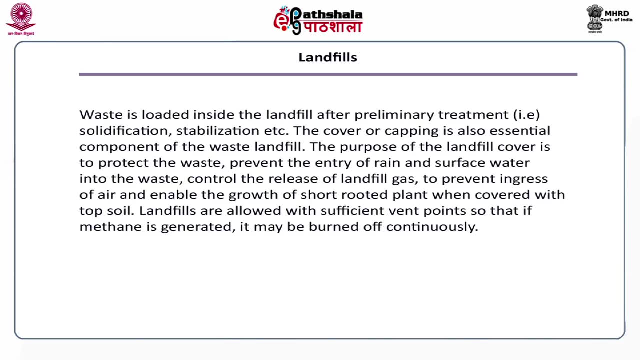 the failure of primary leachate system. Continuous monitoring of the groundwater from the wall will help us to determine the failure of primary and secondary liner system. Waste is loaded inside the landfill after preliminary treatment such as solidification, stabilization, etc. The cover, or capping, is essential component for waste management. The purpose of the 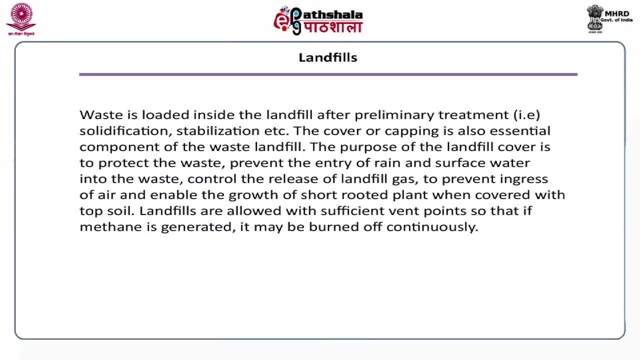 landfill cover is to protect the waste, prevent the entry of rain and surface water into the waste and control the release of landfill gas to prevent ingress of air and enable growth of short rooted plants. when covered with topsoil, Landfills are allowed with sufficient vent points so that, if methane is generated, it 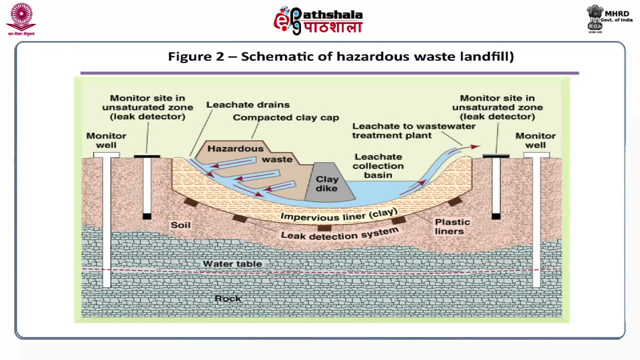 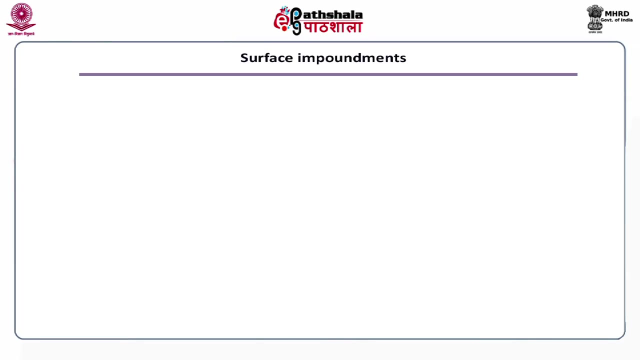 may be burned off continuously. Now here is a figure which depicts schematic of hazardous waste landfill. In this figure we can clearly see monitoring well on either side of leachate collection basin, which is followed by monitoring site in unsaturated zone, Now surface impoundments. 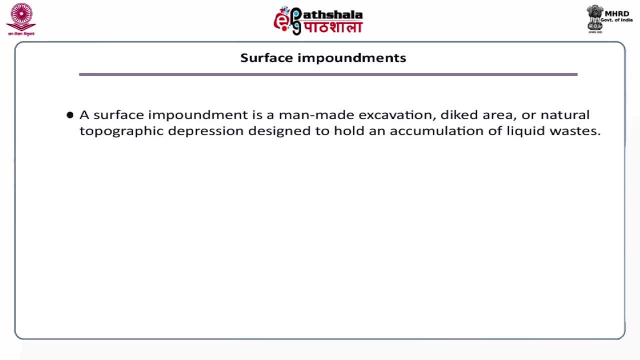 A surface impoundment is a manmade excavation, diked area or natural topographic depression designed to hold end accumulation of liquid waste. The construction is similar to landfill, where the bottom wall function like liner, which is impermeable to liquids. The surface impoundments are also provided with provision for leachate collection. Your 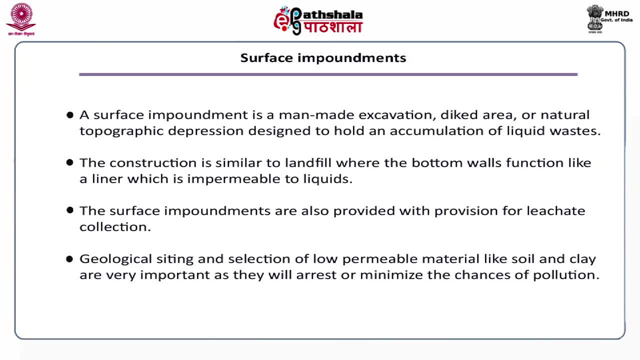 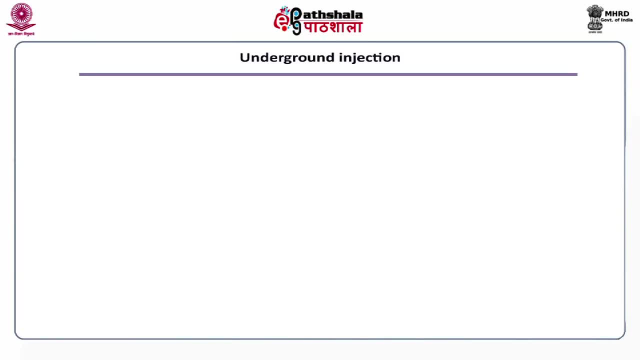 logical citing and selection of low permeable material like soil and clay are very important inỰhich halt production of leachate. So various siding units are were shown here, as they will arrest or minimize the chances of pollution. Now next is underground injection. 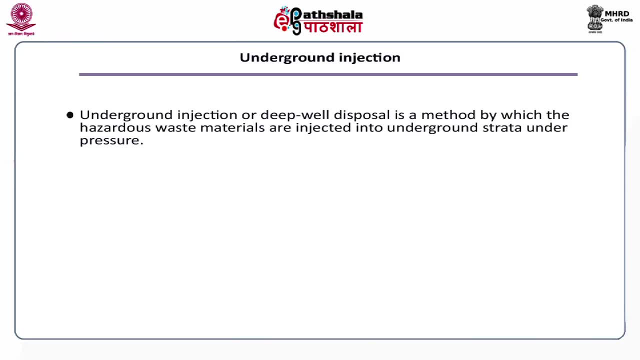 Underground injection or deep well disposal is method by which the hazardous waste material are injected into underground strata under pressure. The underground strata must be impermeable and separated from the aquifers. During this process, the chance of chemical reactions with waste constituent and mineral